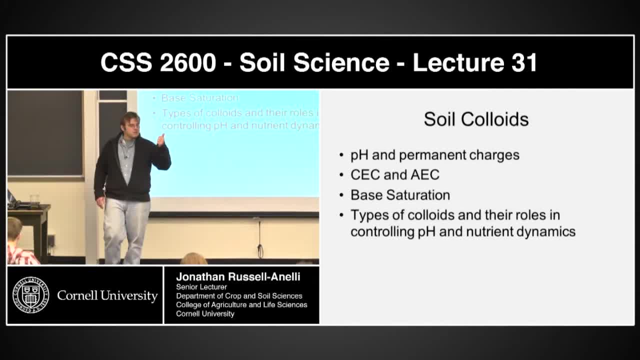 We talked about the. We talked about the phyllosilicates, the amorphous, the non-silicate, the non-sheet colloids. We talked about oxides And then we talked about the organic colloids. We talked about the organic colloids in the sense of colloids. 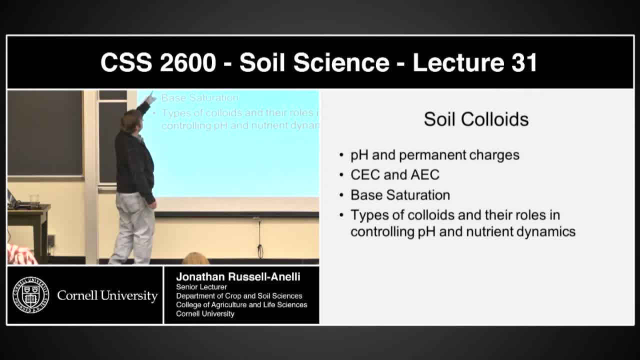 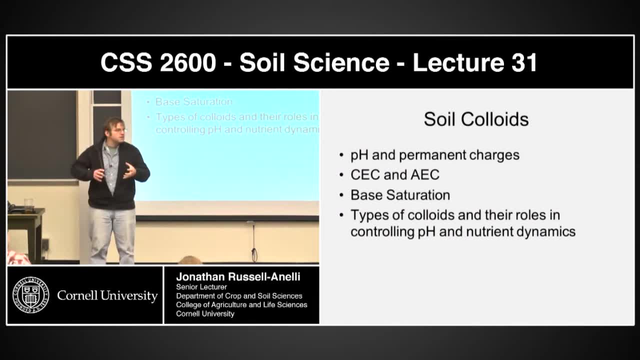 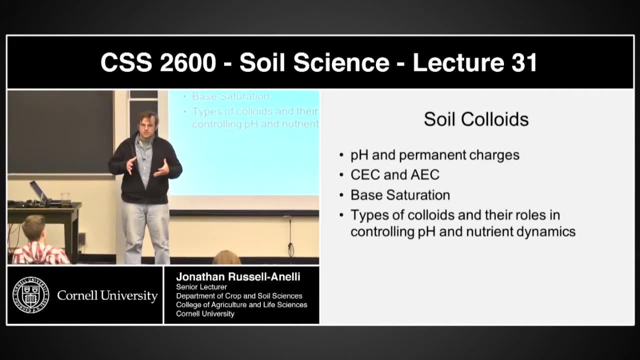 not in the sense of organic matter. Now, when we talked about those things, we were very much talking about this issue of the structure: what makes this material, what is it made out of, and also how that structure impacts the issue of the edge, the surface areas. 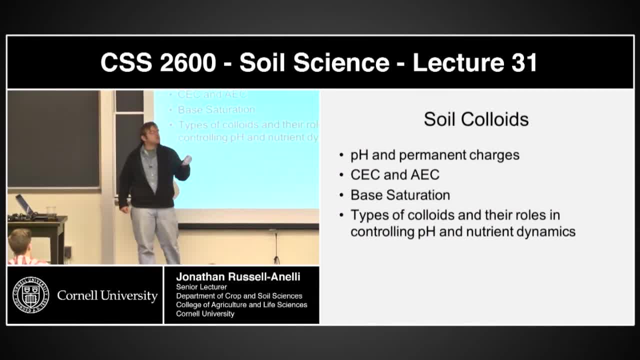 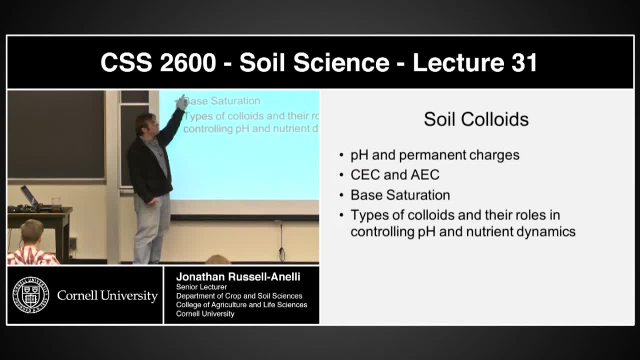 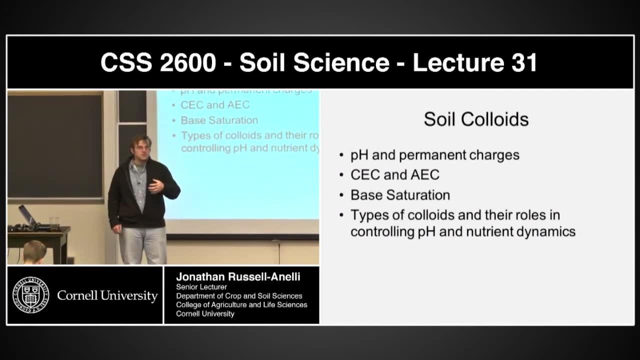 And that's when we started talking about the issue of permanent charge as well as the pH dependent charge. On that note, that segued right into this issue of CEC and AEC, Because of the isomorphic substitution, because of the structural arrangement of these phyllosilicates. 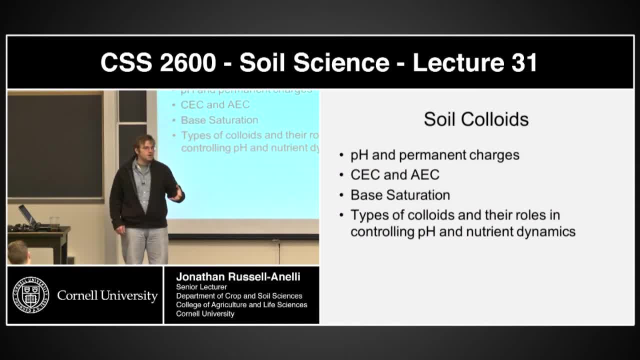 as well as the other type of colloids. what is the charge associated with these particles? Let me take a step back Again. when we talk about colloids- and we talked about this initially- when we're talking about colloids, colloids is a description of a size. 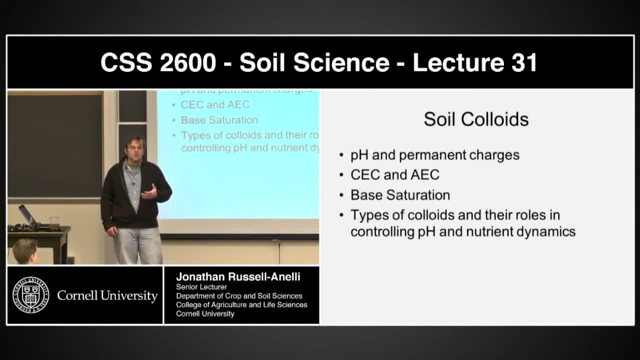 There are a lot of different things that are of that size, But colloids are what size? Basically one micron and smaller. So this is why surface area is so important. Now, once we got done with talking about cation exchange, we started talking about this issue of base saturation. 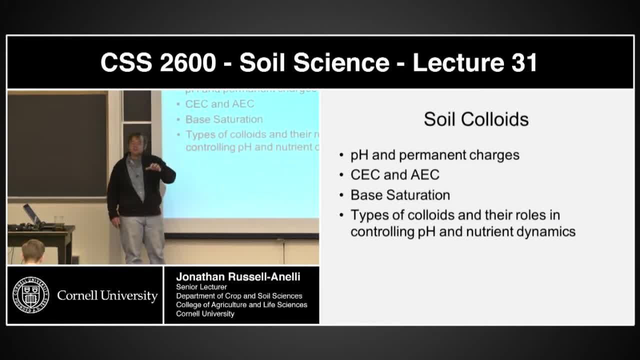 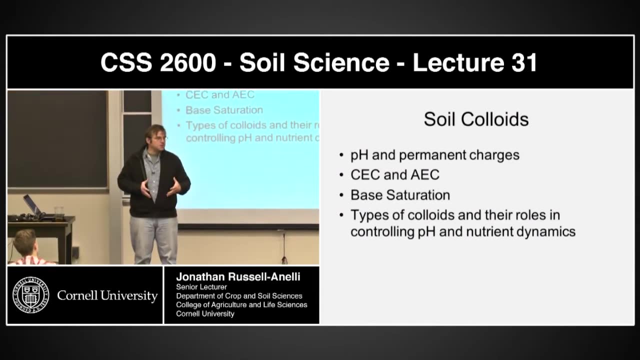 Base saturation is a measurement of how much cations are on that cation exchange site. You can have a rather large cation exchange capacity, the capacity, the whole number. but that doesn't necessarily mean it's all occupied by bases. It could be occupied by protons or aluminum. 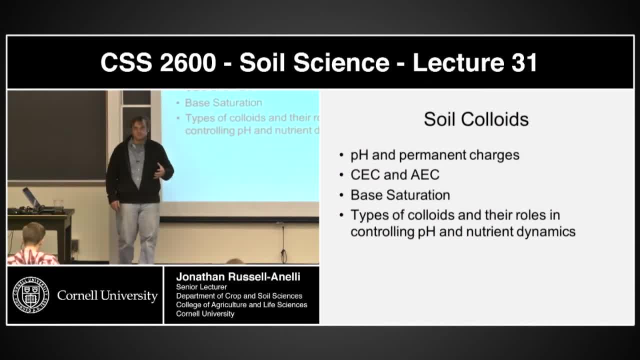 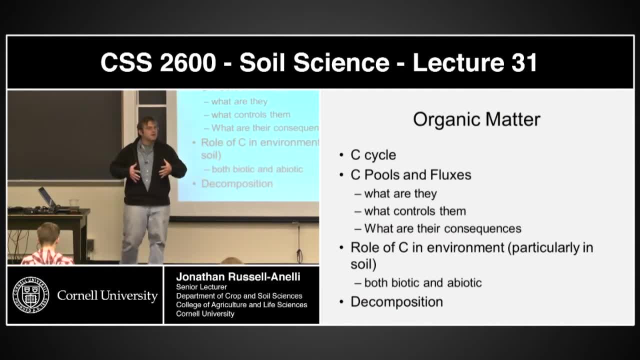 And then this was the segue into what is the pH. The next thing we talked about was organic matter and we started talking about organic matter. I just wanted you to get a sort of concept of what organic was and sort of the organic cycle, the carbon cycle. 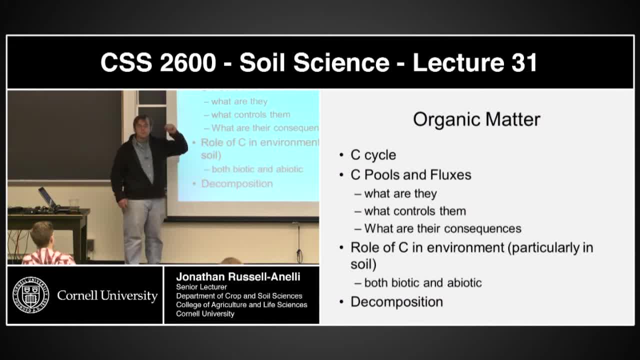 So we talked about the carbon cycle. We talked about the carbon pools and their fluxes, what they are, what controls them and what are their consequences. We then went on to start talking about the role of carbon in the environment, particularly in the soil. 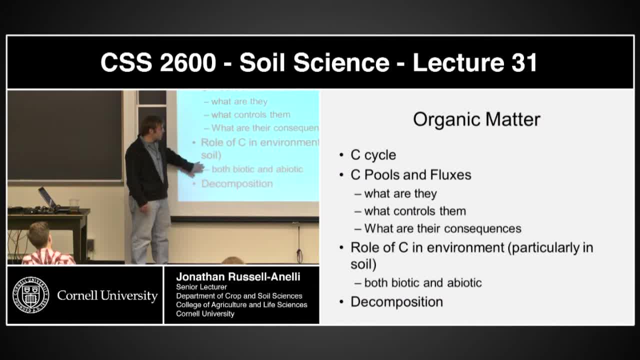 Okay, But we also talked- when we were talking about this role of carbon, we were talking about biotic and abiotic activities, things that were going on, but we also started talking about decomposition. Now, at the same time that we started talking about decomposition, 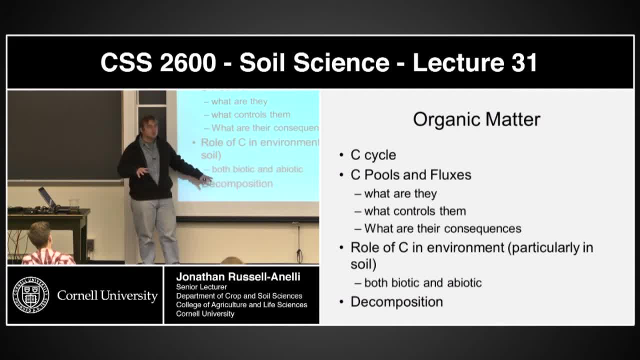 this almost segued into soil ecology, because we started talking about how that decomposition occurs, the issue of location, structure, all those types of things. But we also talked about the nature of the organisms that were doing the decomposition, the sort of the artifact of the nature of that carbon. 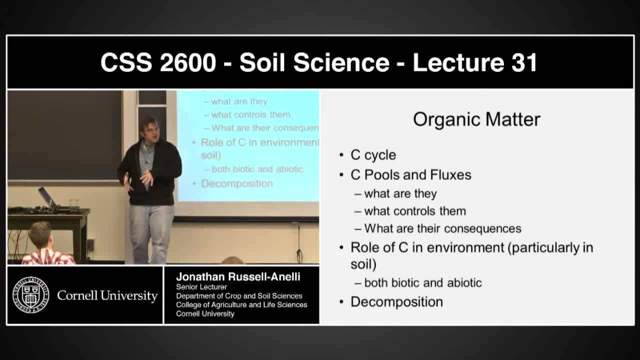 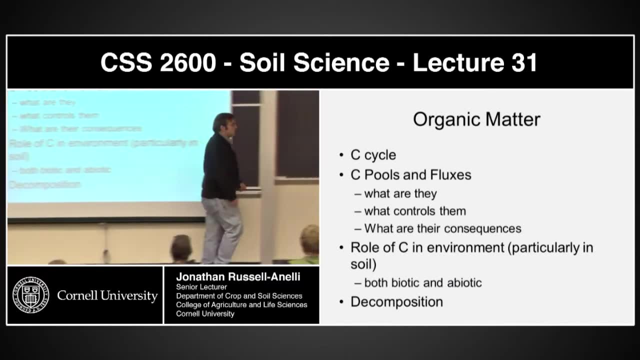 and its effect on the organisms that are doing the decomposition and the artifact of the decomposition by the organisms on the carbon itself. Right, Do you guys remember that whole conversation? So when we start talking about decomposition, we're basically- and we'll talk about this- in the context of an aerobic system. 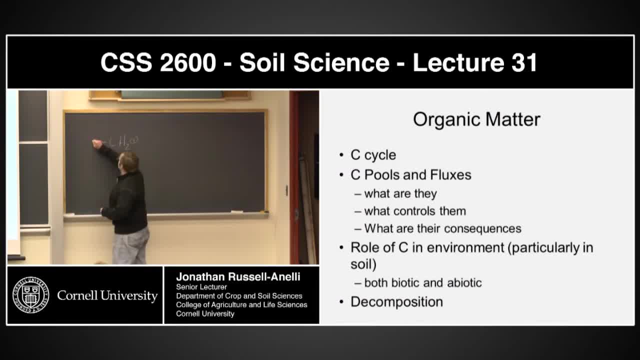 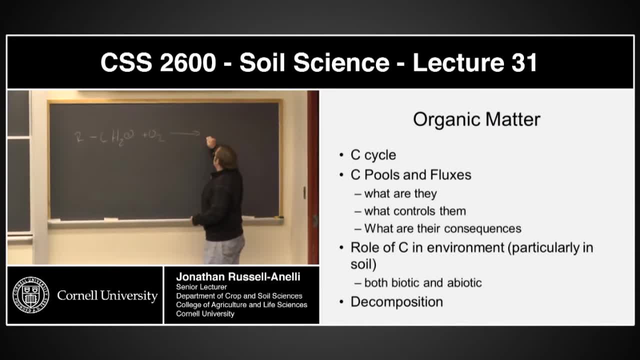 but we have an organic molecule, whatever it happens to be, Okay. A repeated organic molecule structure: Okay. And in the presence of oxygen generally. this is what we most, most people, think as sort of the decomposition process. Now, the reality is there's a lot of other things going on here. 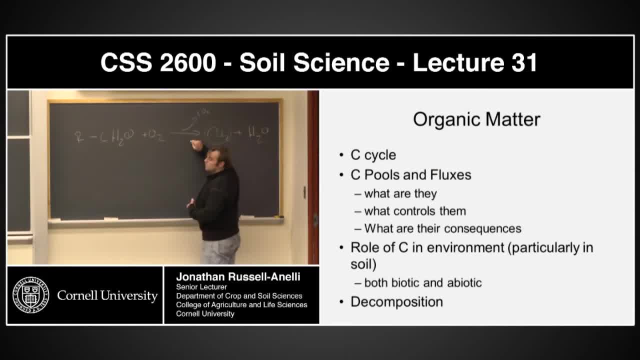 We're certainly going to be blowing off CO2, which is this- but we're also going to be getting energy and we're going to be getting nutrients out of this system. I mean, why are we? why are we eating? It's not to produce this. 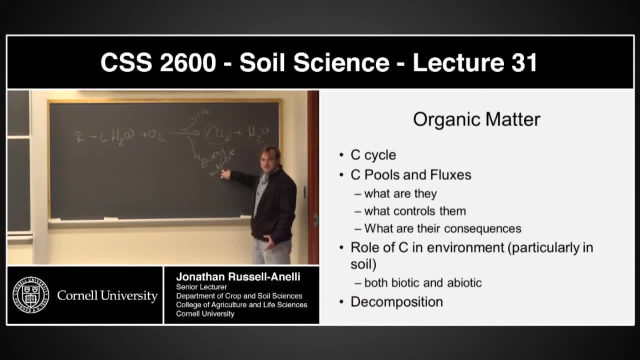 It's to get this Right. Does that make sense? Okay, So the nature of this molecule and the environment in which it is in is going to have a huge impact on what you get out of it, And that was sort of the segue from organic matter. 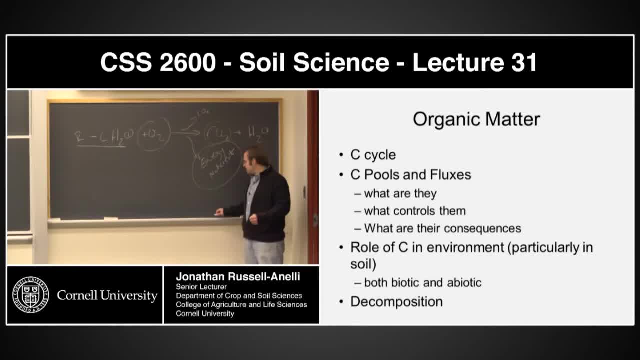 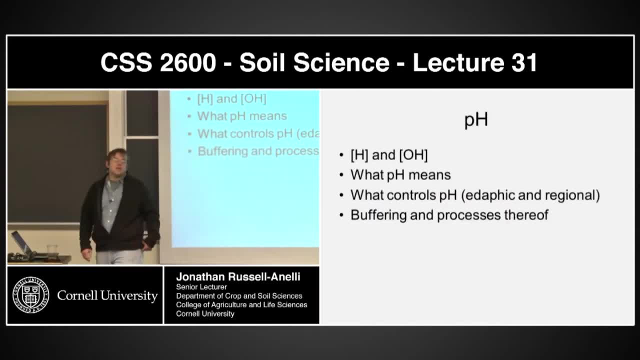 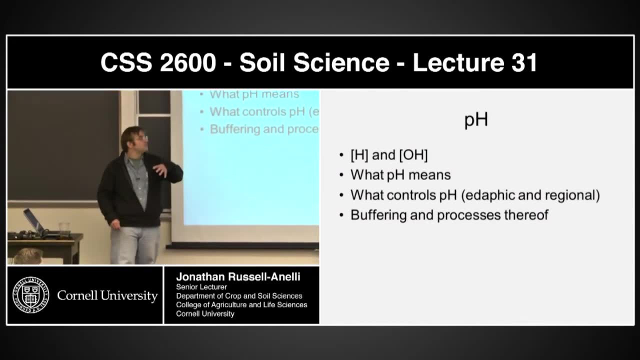 to soil ecology. Okay, The next thing we talked about was pH, And this was sort of to close out this sort of nutrient end of the spectrum and sort of leg us into nutrients at the same time. But we started with talking about what 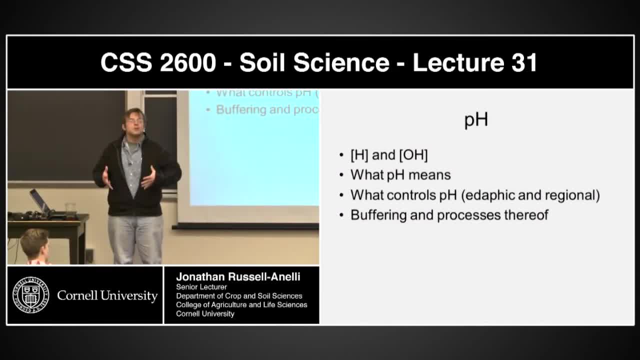 well, what is pH? You know it's this issue of proton concentration, this issue that water disassociates at a constant Okay, And that disassociation depending upon what is more predominant, from that disassociation in the soil solution, you're going to get an acidic system. 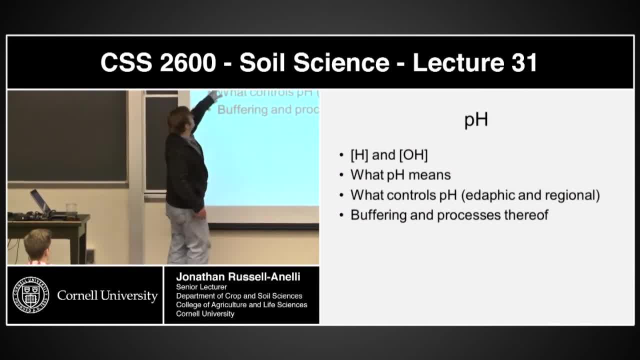 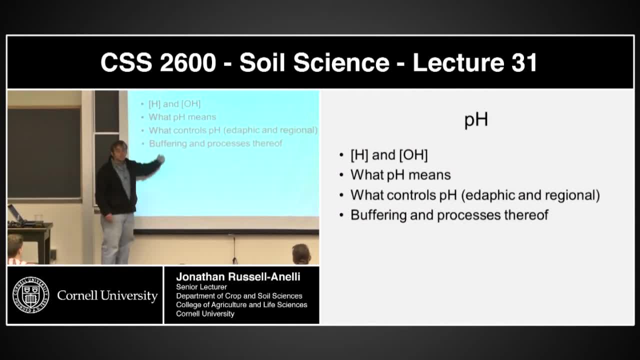 or an alkaline system. Okay, And so we talked about the difference between what hydrogen is and what hydroxide is, and the issue of pH versus pOH. Okay, In essence, we tried, we talked about what pH means. Then the next thing we talked about was: 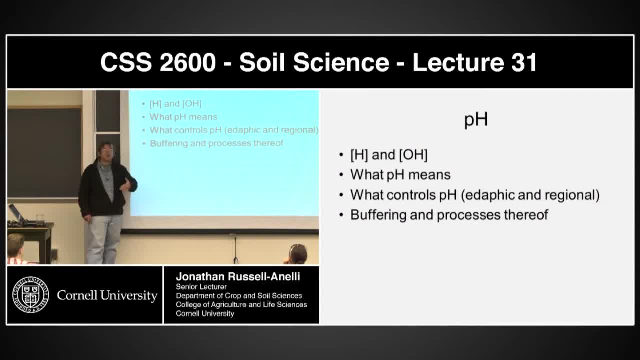 what, in fact, controls that pH and, in turn, what pH controls. And then, finally, we ended up with talking about buffering- how pHs are modified in the environment- Okay, How they're buffered, in essence- and the processes that drive that buffering and the processes that control that pH. 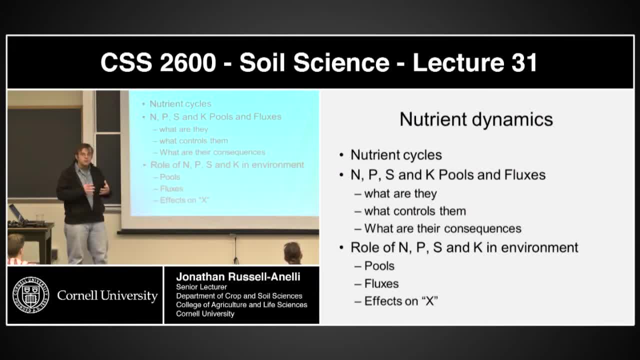 We then went into nutrient dynamics. Okay, We started with nitrogen, but we basically went through all of the different- well, not all of them- four of the different nutrients. The context here is we're looking at a nutrient cycle that's totally controlled by microbial populations. 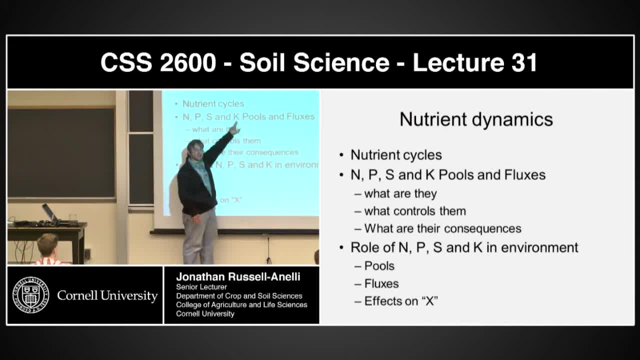 or an ecological system to a system where there's basically no ecological controls. I mean, this is always in its ionic form. It's not truly. it's not being put into biomass. It's always in an ionic form, whether it's in the soil solution. 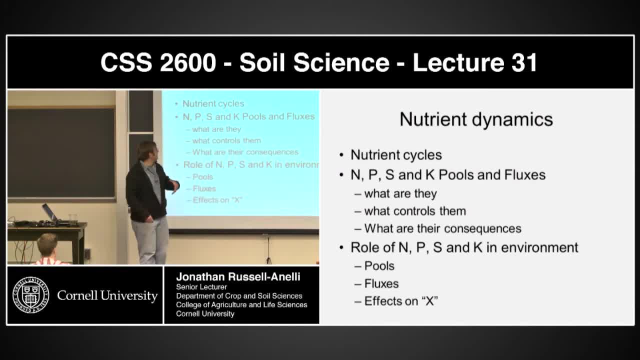 whether it is in the biomass of an organism. Okay, We talked about what they are, what controls them. Okay, I hear the pools, the fluxes and what are their consequences. What is the impact of these pools and these fluxes on the larger environment? 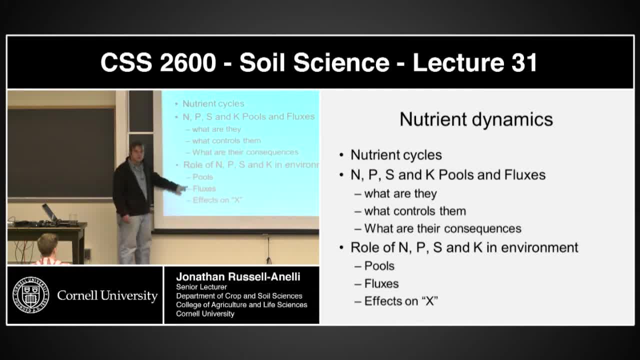 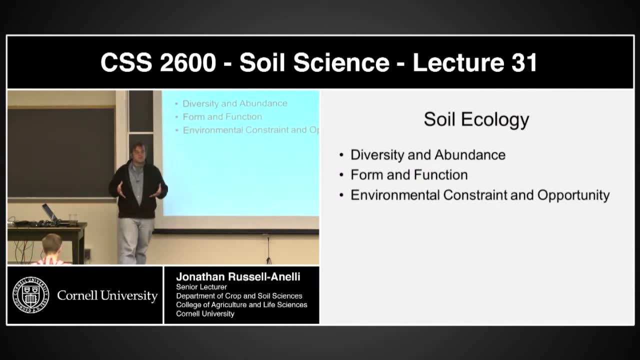 Okay, And that was this whole section that we talked about. This was basically the meat of each one of these lectures. Okay, The last lecture section that we had was soil ecology, and this is where we started with classification, but this quickly slipped right into this issue. 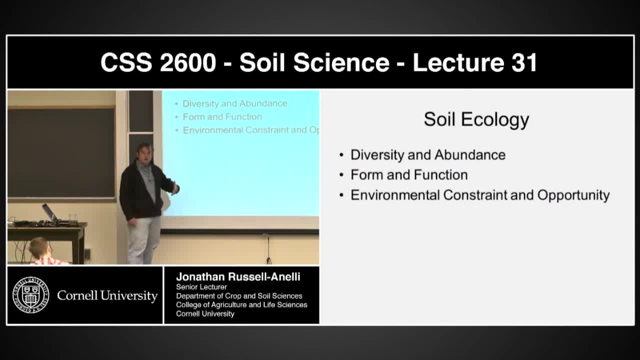 of diversity and abundance, the form and function of those organisms, and then the environmental constraints and opportunities. Okay, That, in a nutshell, was what we talked about over the last five weeks-ish kind of-ish. All right, So what I'd like to do today? 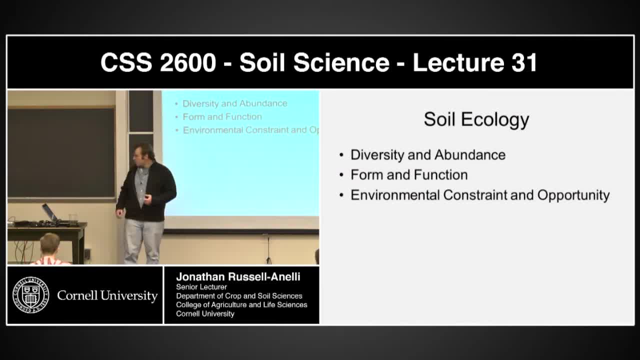 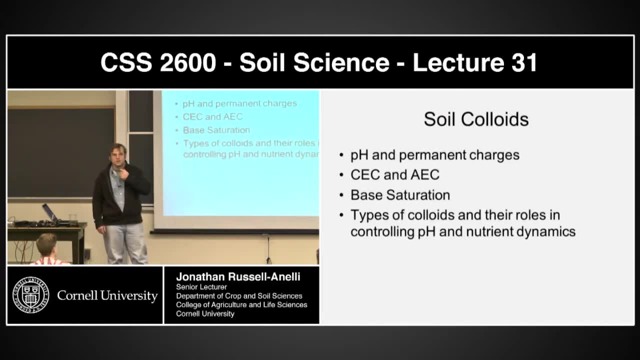 now is open it up to you guys, and I want to open it up by opening it up to soil colloids and see if we have any questions on soil colloids in particular. Go, Yeah, they do. Okay, So the pH dependent charge. 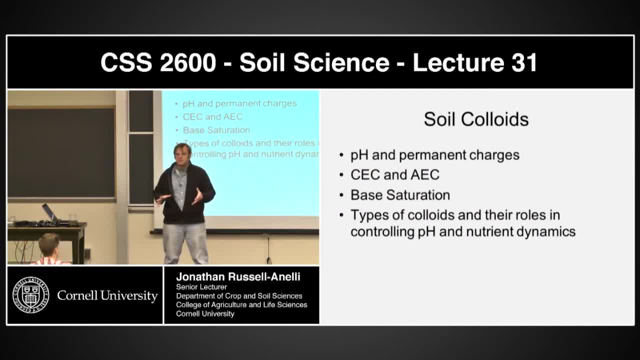 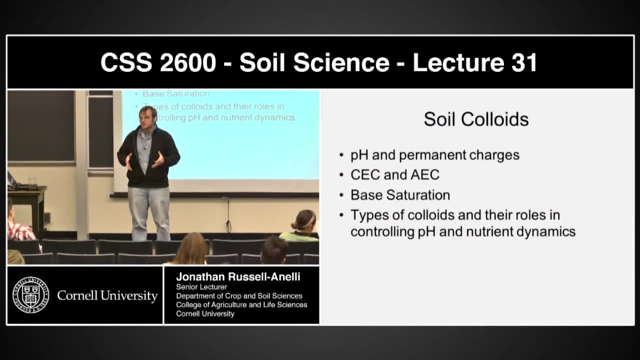 So we have a permanent charge. Everybody sort of get that, the idea that these colloids, these small particles, depending on what the kind of material they are, they have a permanent charge. Okay, That's associated with their structure, But that structure. 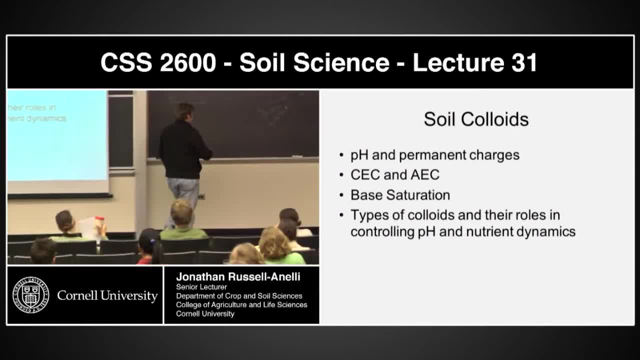 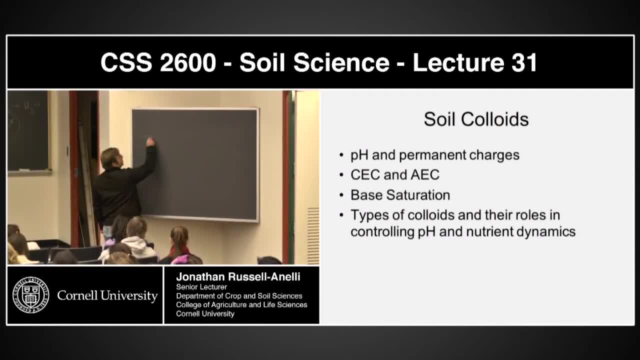 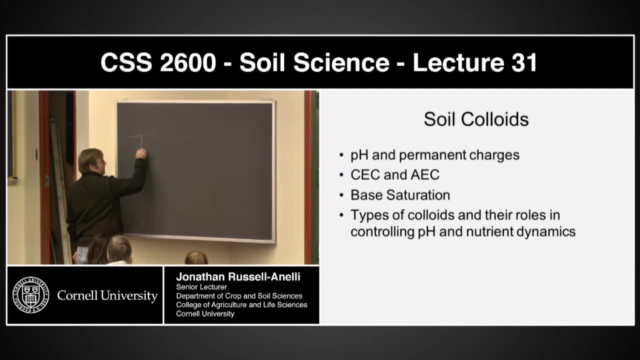 depending upon where it interacts with the soil solution. basically, all of these colloids have whatever that material is at the edge of. you know, it could be an organic molecule, it could be a clay molecule, something like that. All of them basically have this hydroxyl group on the end. 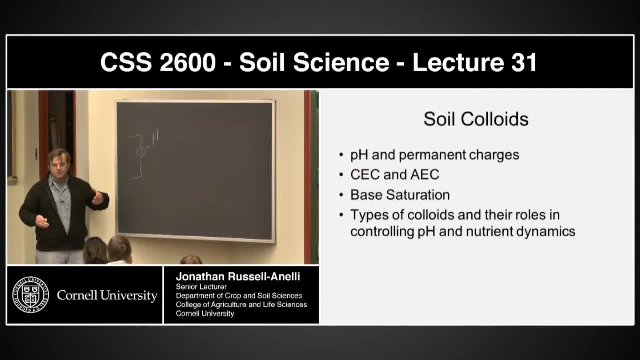 Right, This is the edge. So from a phyllosilicate you can imagine. I have a repeating structure that's looking like this. You know, I have a tetrahedral sheet, tetrahedral sheet and an octahedral sheet. 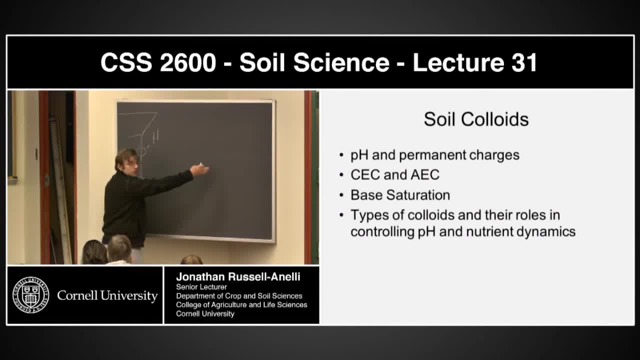 Well, this is that edge. That edge is imperfect because it doesn't continue. So I have the oxygens that binding the aluminum and silica together, And they do not have another aluminum silica over here, So they're exposed to the soil solution. 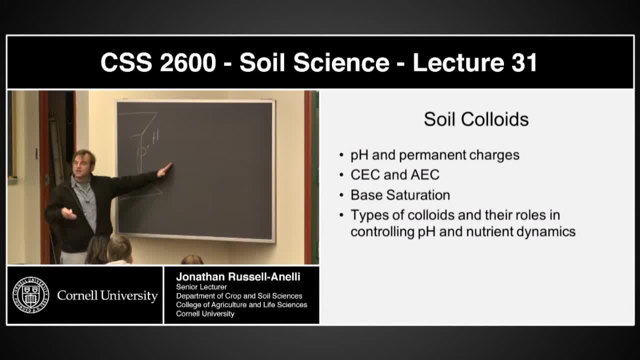 And at that, oxygen- because it's exposed to the soil solution and it doesn't have a silica or aluminum that it's binding to- is going to be interacting with the protons that are in that soil solution, making, in essence, hydroxide. 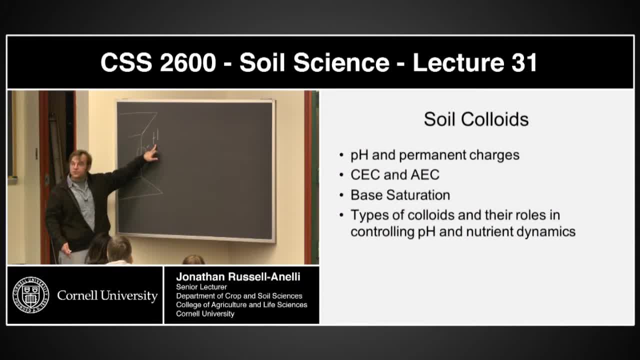 Okay. Now this hydroxide is not part of the structure, which means it can interact with the soil solution. Now what's going to happen if the pH starts to rise? That's going to equal: I'm going to have an increase in what? 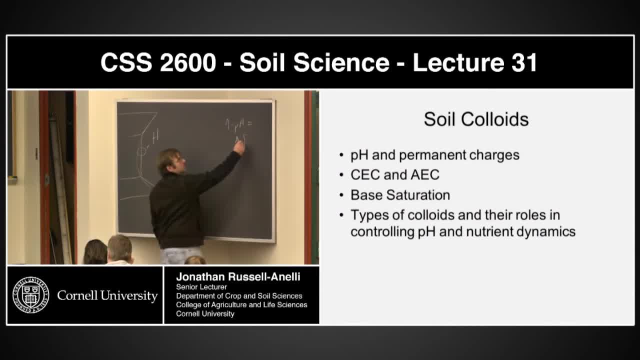 The concentration of what. Okay, if that happens, that OH is going to be going into solution and it's going to react with this proton. pull it off and make water, Because it's taking this away. this has a positive charge. 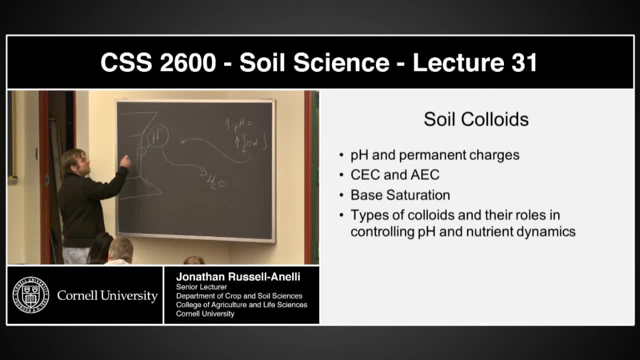 So it's going to create a relative increase. This is already negatively charged, but what it's going to do is it's going to increase the relative negative charge of this calloid. So, in essence, it's going to increase the cation exchange capacity. 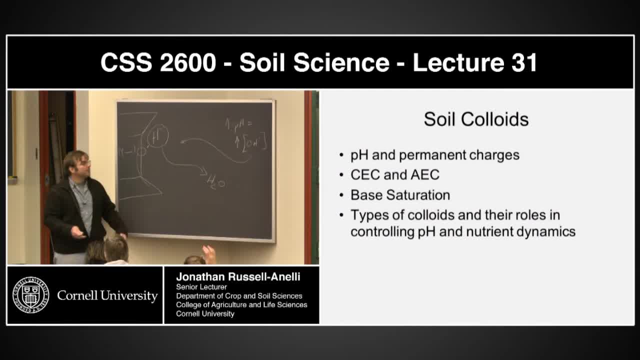 Does that make sense? All right. Now what happens when we start adding protons to this soil solution? The pH is going to start going down Right With the increase in proton concentration. This proton is going to start acting, reacting. 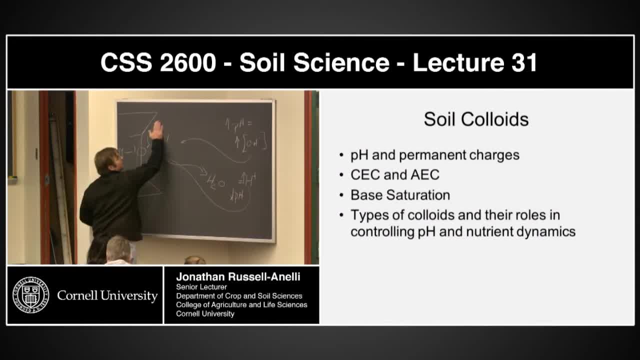 with this hydroxide, this oxygen. Okay, there's no proton here. now, right, That proton went with the water. So if I start increasing the proton concentration, those protons are going to start rebinding there. What's that going to do to my CEC? 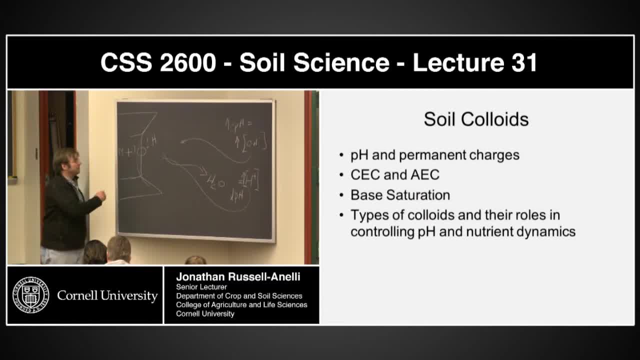 It's going to make it more positive right? My cation exchange capacity is the ability for this calloid to hang on to positive charges. So if this gets more positive, its ability to hold on to positive charges is going to be going down. 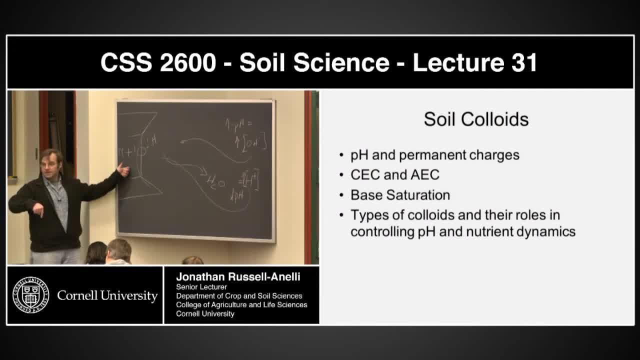 Right, Does that make sense? And if I continue to drive this pH down, I potentially can hold another proton here which is going to make it even more positive, which is going to drive my CEC down even more. But what is it going to do to my AEC? 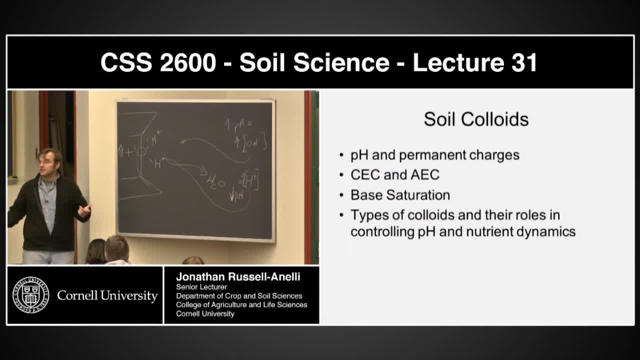 my anion exchange capacity. It's going to increase it. So as the pH goes down, my CEC goes down, but my AEC goes up. As the pH goes up- an increase in this- my CEC is going to go up. 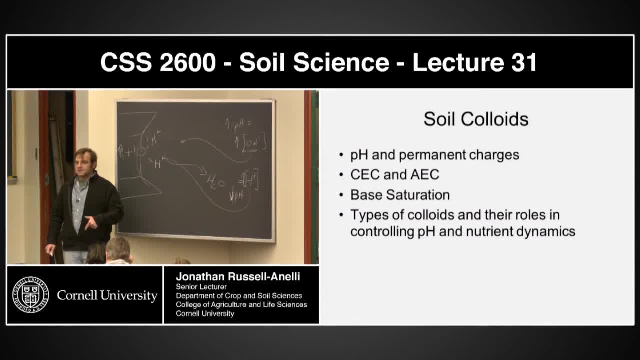 but my AEC is going to go down. Does that make sense to everybody? Because what I'm doing is I'm changing this relative charge in the calloid And it's very temporary and it's totally controlled by the pH. It's not structural. 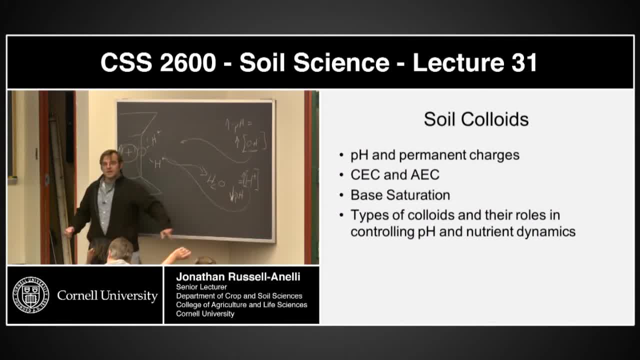 Right, Cool beans, Okay, Go. In this case, this is a buffering reaction. Okay, In a sense, because what's going to happen is right now we're just looking at the protons, but as I start changing these cation exchange capacities, 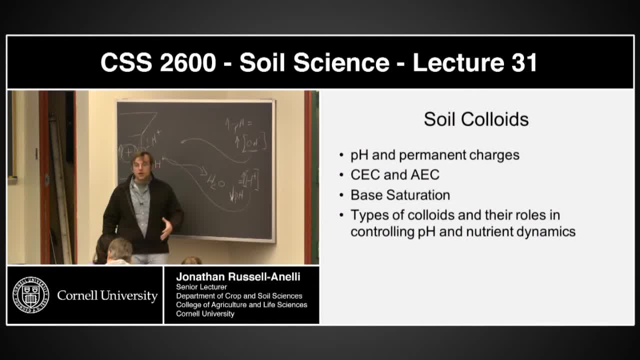 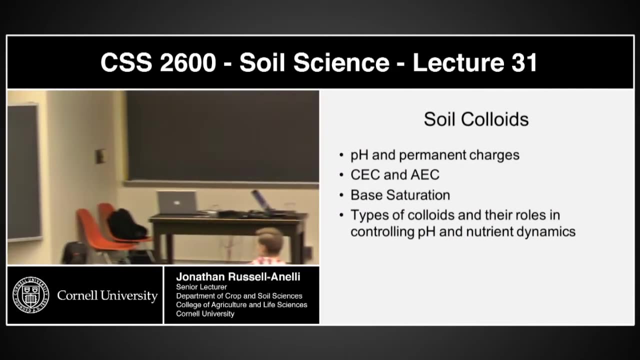 I start putting more and more protons in solar solution. the permanent charge as well as the pH dependent charge. those charges are going to have something associated with them, right? Let's use this board over here. Okay, so here's my calloid again. 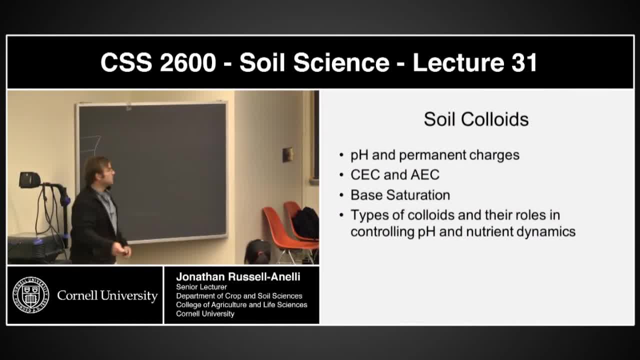 Okay, And we're going to start with a pH that's high. Okay, If I have a high pH, what does that mean to my CEC? It's larger, right? Okay, if I have a larger CEC, it's going to be more negative. 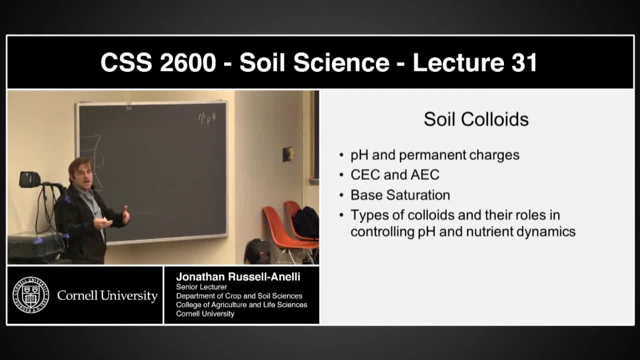 Now, if that's the case, it's going to be holding on, even if it's not as long as I have some CEC. it's going to be holding on to bases, All right. So let's imagine that's a calcium. 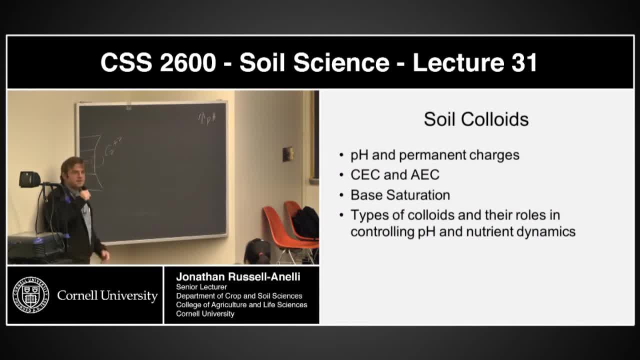 that's being held here, Right, All right. So what happens when we start lowering the pH? Okay, I start lowering the pH. I'm going to start seeing. if I start lowering the pH, I'm going to start seeing an increase. 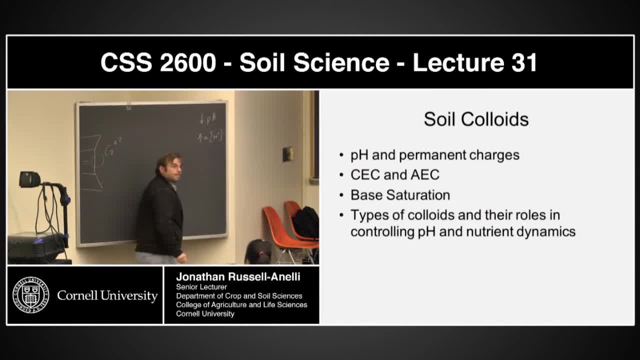 in the concentration of protons Right. What are those protons going to do? They're going to start, they're going to go into solution and they're going to start competing with this cation exchange site. Now, this happens to be plus 2.. 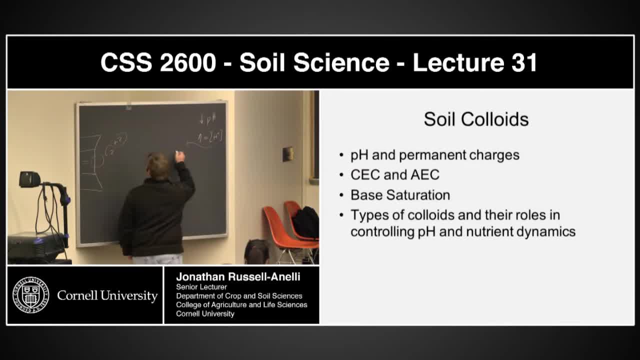 Proton happens to be plus 1.. So if this proton goes over there and it hits a plus 2, it's probably not going to do anything. This plus 2 is probably going to hold on, But as I start increasing this concentration, 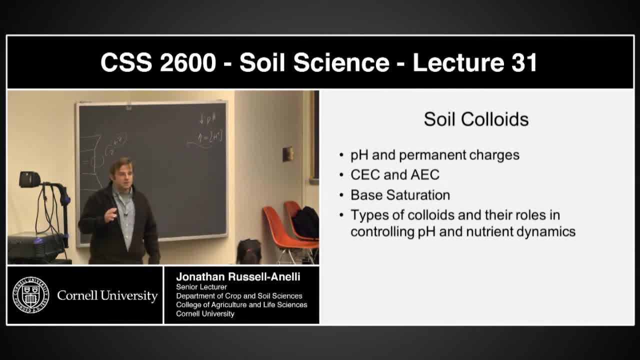 do you guys remember the cation exchange rules? Mass action, right? Okay, I'm going to start getting mass action because I have more protons. I start moving enough defenders against that offensive soccer player. sooner or later they're going to be able to take the ball away. 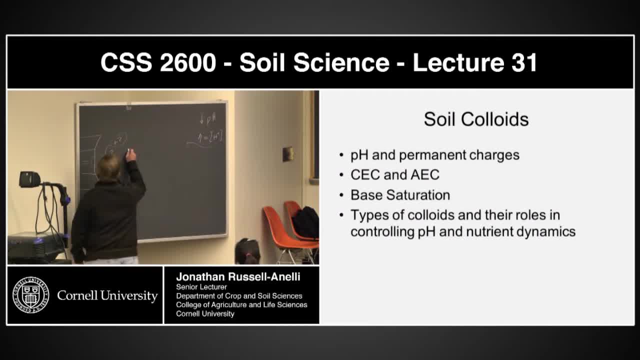 Right, Okay. So if I take off protons, sooner or later they're going to knock this cation off. But in the process of knocking that cation off, I'm getting two protons here. What's that going to do? 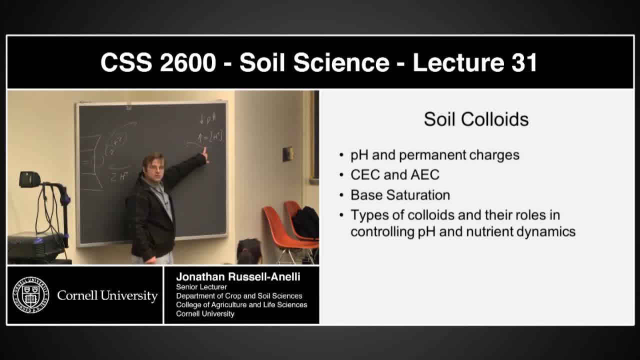 to the relative concentration of protons that are in the soil solution, It's going to reduce it, So in essence it's going to buffer the proton concentration. Does that make sense? Because in the process of knocking this calcium off, it's taking two protons out of the soil solution. 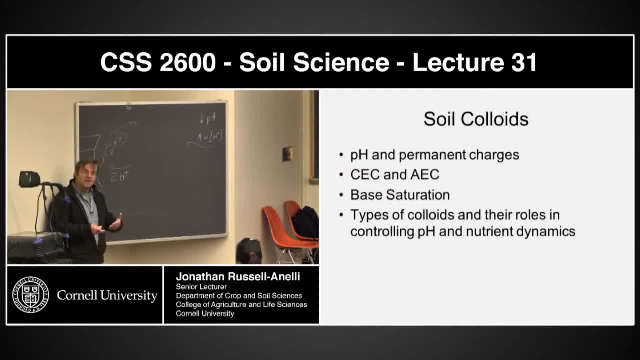 If I take protons out of the soil solution, I'm in essence raising the pH of my active pH Right, So it's a buffering reaction. all at the same time Cool beans- I don't know if that answered your question. 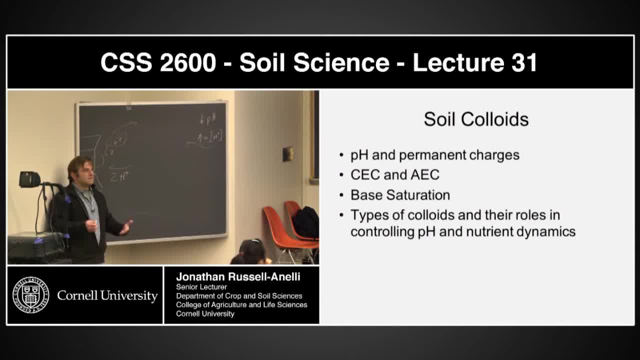 Kind Is that the whole. that's the only way they can go through the buffering. This is the kind of buffering that happens in the middle. Remember, we have buffering that happens at high pHs. that has to do with calcium carbonate. 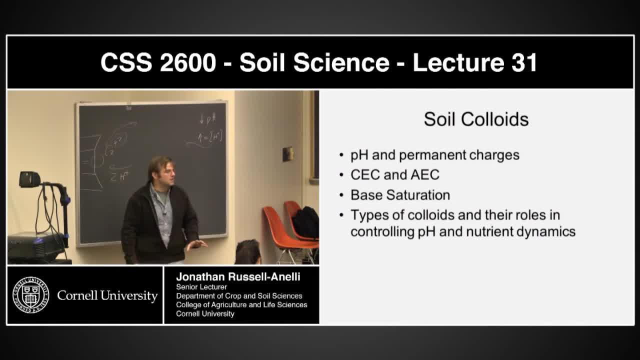 and then we have buffering. that happens at low pHs, which happens to do with aluminum hydroxides, gibbsite, Right, And those are things that you guys should know. Hint, Okay, other questions on this one. Do we have to know? 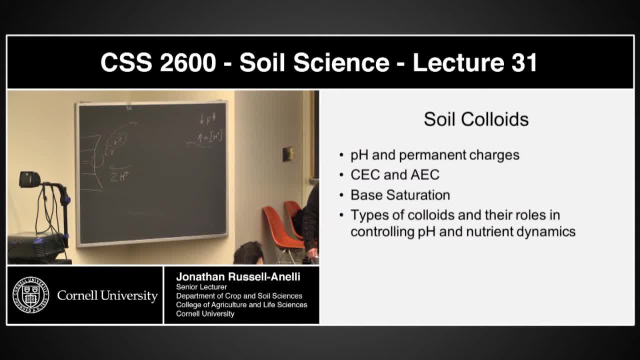 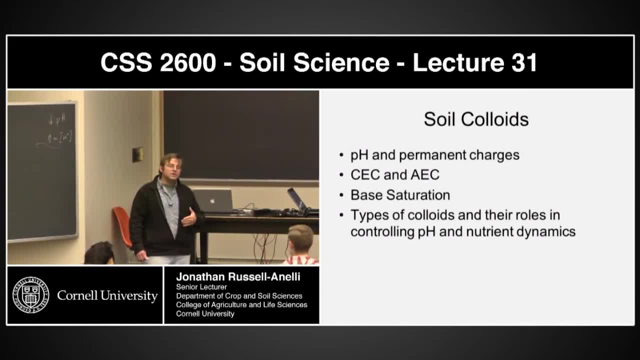 all the exact types of colloids, like smectite, and that they're two to one or whatever. So the question is: do I need to know all the exact types of colloids? I want you to know the four types of colloids. 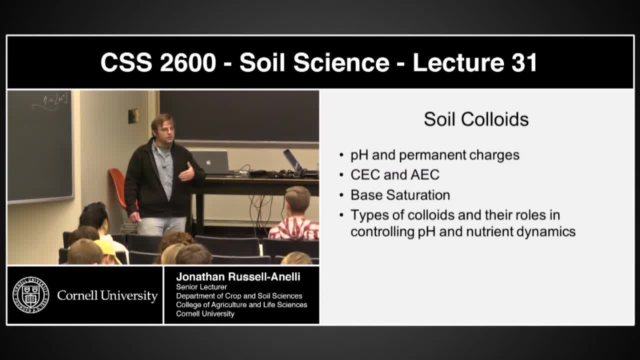 but I don't necessarily want you to know the specifics of each type of colloid. You need to know what a phyllosilicate is. You need to know what an amorphous colloid is. You need to know what an organic one is. 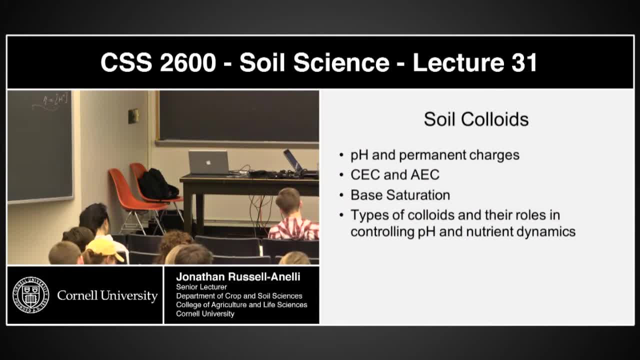 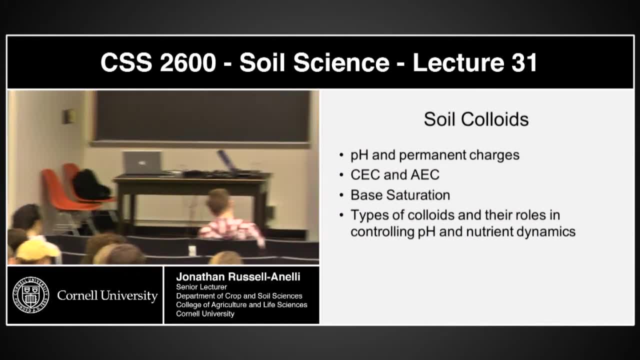 You need to organic colloid. You need to know what an oxide is- Okay. you need to know what they are- Okay. But you don't need to know all of the two to ones and the one to ones and the two to one to ones. 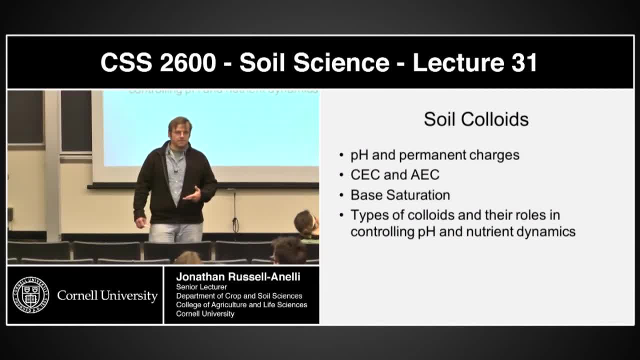 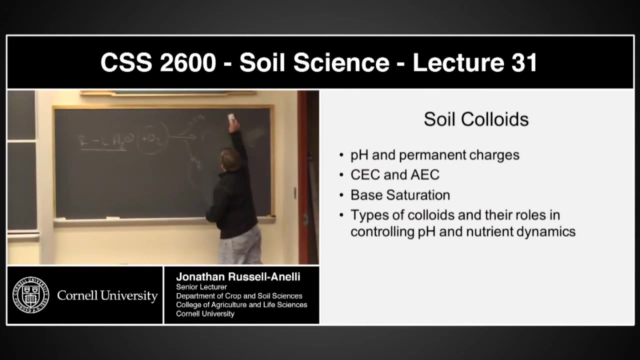 of the phyllosilicates. Okay, All right. Next question: We feel does everybody feel comfortable about this one. We'll move on to the next Good question. Okay, So what's the difference between the CEC and base saturation? 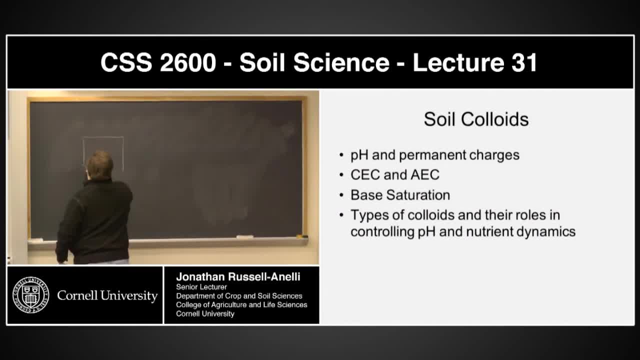 So if I have a colloid, okay, it's going to have a certain charge associated with it, And forget about whether it's pH-dependent charge or a permanent charge. That colloid is going to have an absolute amount of charge, positive as well as negative. 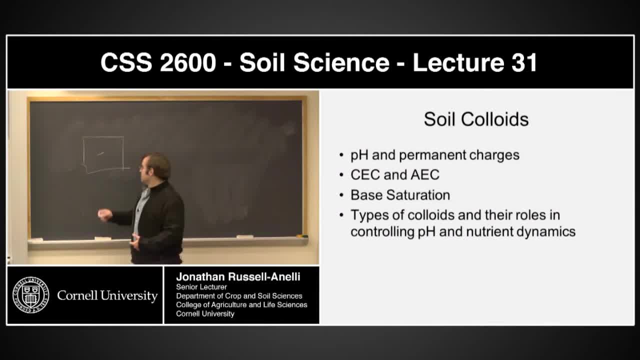 Okay, If it's a negative charge, that absolute amount, and let's imagine that it is 100.. Okay, that means it can hang on to 100 positive charges. CEC is a measurement of the absolute charge, It's not a measure. 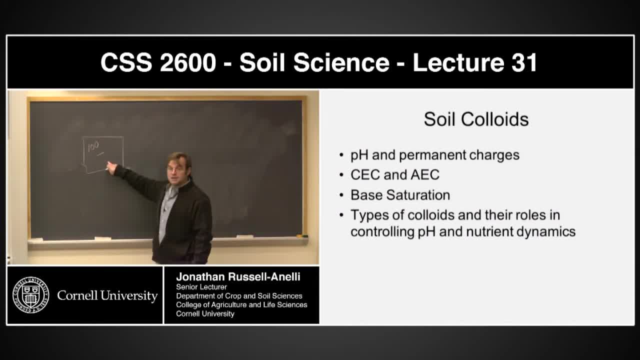 about what is in fact held by it. It's just its measurement. It's got a negative 100, negative charges. That's it. Base saturation is a measurement of how much of this 100 is occupied by bases. Okay, So if I have 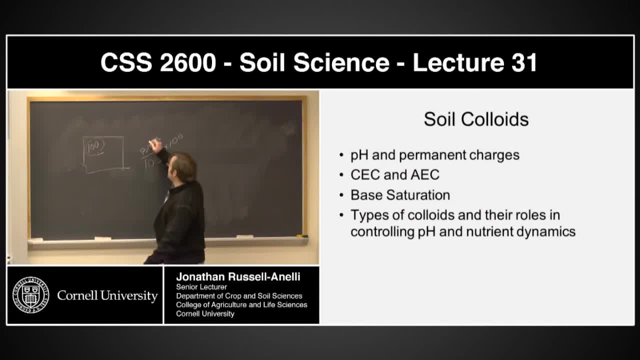 of these 100 charges I have 50 positive charges that are attached. that means I have 50 over 100 times 100 for the percentage. That means I have a 50% base saturation. Does that make sense Now, as those bases come off? 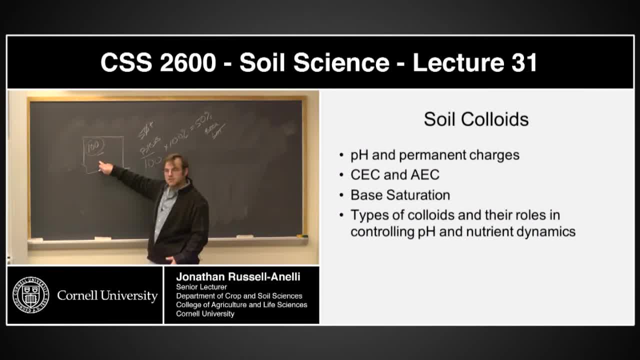 I'm not changing my CEC, I'm just changing the base saturation Right Go. So, CEC, that charge is reflected just at the surface. The CEC is the charge that's reflected. It's the exchangeable. It's the exchangeable. 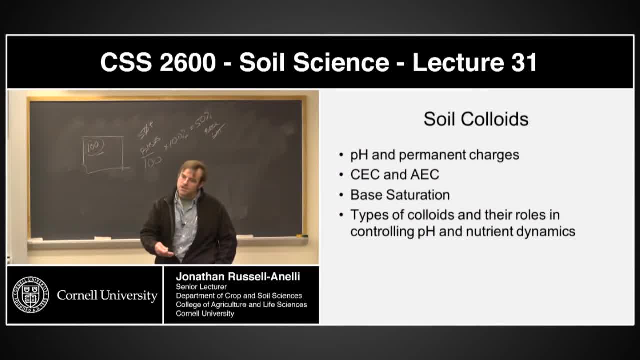 So it's reflected at the surface, but the charge itself may come from internal isomorphic substitution. But okay, so here's my magnet Right. The isomorphic substitution may be inside, but the interaction is going to be at the edges. 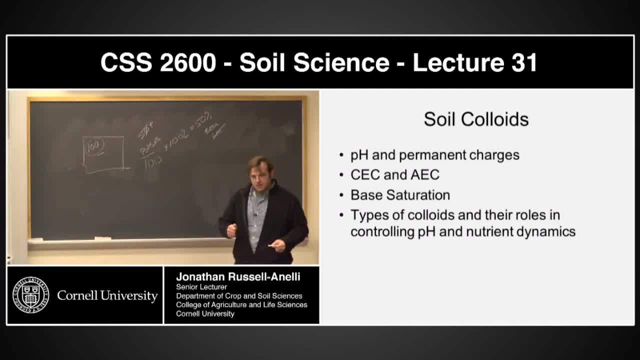 Okay, does that make sense to everybody, Sheila? Like, from a practical standpoint, is CEC like something based on, like, like the- you know the amount of sand and like what is it touching? Okay, so from a practical sense, 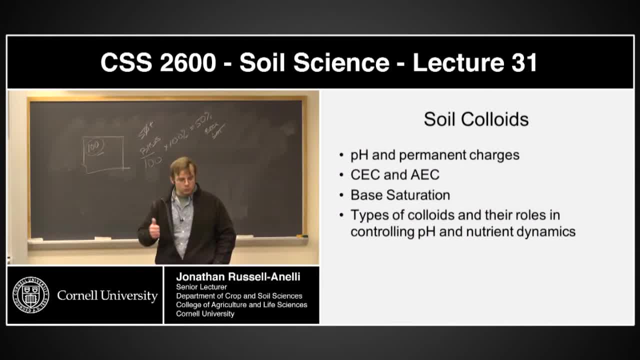 CEC is measured in two ways. One is we sort of have a rule of thumb where sands we look at a sand, a silt and a clay. Now the reality is clays are very different From a laboratory sense. we basically measure this. 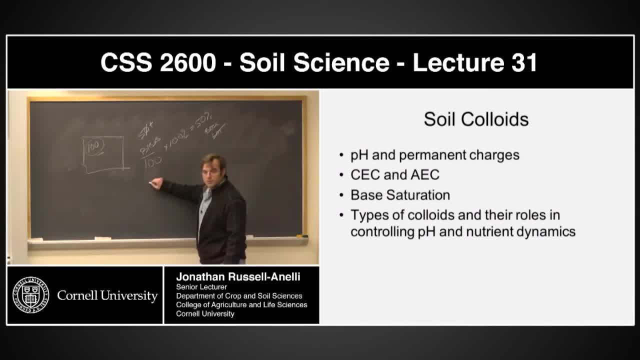 by putting. that was that whole soil solution thing, where we put a material in a solution, okay, and we saturate it with something. It could be an ammonium, you know, or a potassium or something like that. We saturate. 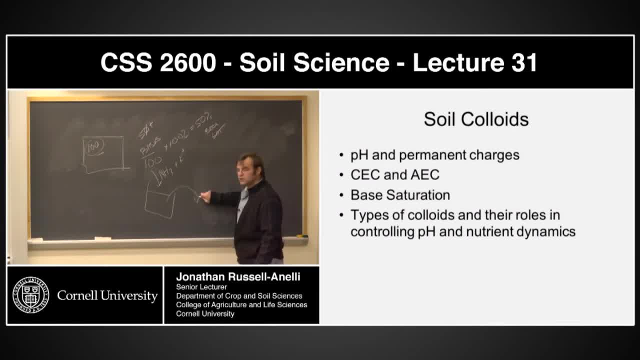 we drive everything off, and then we take that same solution with the soil in it and we add something else and we drive everything else, and then what we do is we measure the ion that we used in the first place and it will tell us. you know. 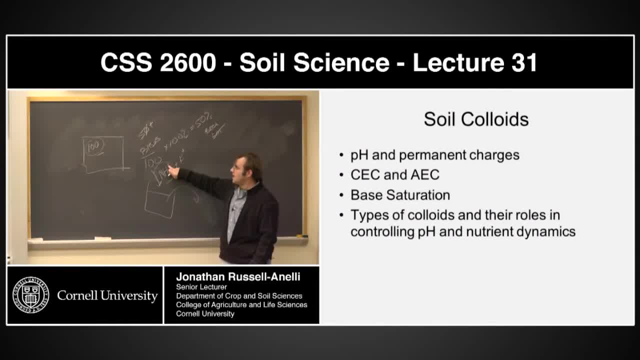 this is a positive charge, and I have 100 of these. I have a base, a CEC, of 100.. This kind of measurement doesn't tell me what my base saturation is, though It tells me what my CEC is. It will tell. 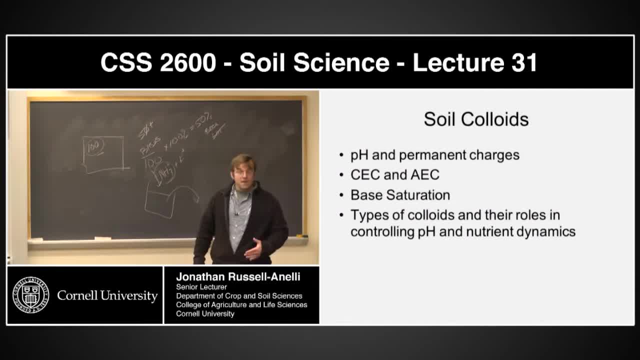 I mean from a potential standpoint. if you have a sand versus a sand and you have a, you know- a sand versus a clay right off the top of your head, you should, if I ask you, which has got more CEC? 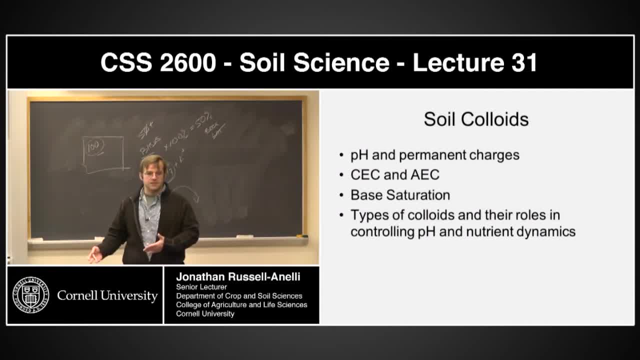 with little thought. you guys should think: well, the clay is going to have more CEC. Well, for a lot of reasons. first off, with clays you're starting to see more and more isomorphic substitution, more charge. 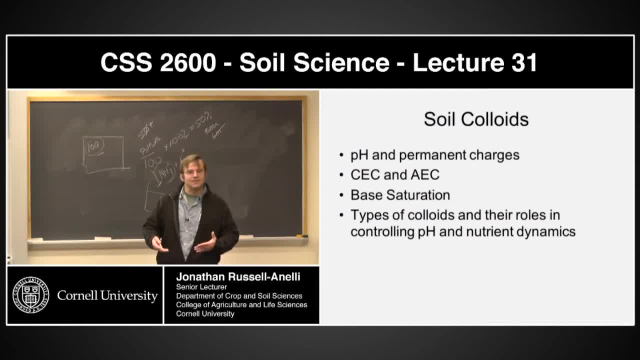 but also I've got a lot of more surface area, a lot of more, a lot more surface area. Right Go. What is isomorphic substitution? Say that again. What is isomorphic substitution? Isomorphic substitution is when we're talking. 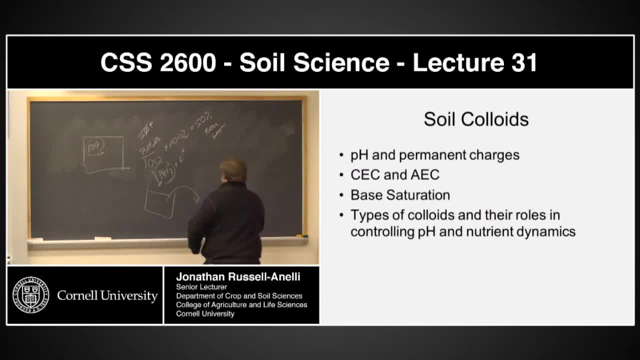 about the. when we're talking about this isomorphic substitution is the sort of the, the genesis of the, of the structure itself. So we start with these tetrahedral sheets, and so this is the classic two to one mineral. 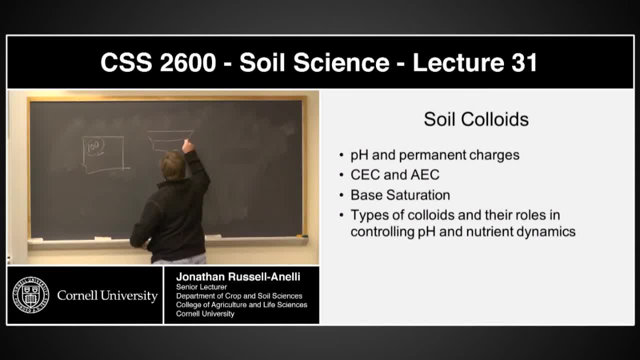 two tetrahedrals and one octahedral. Okay, Well, the tetrahedral, the base structure is a silica and the octahedral, the base structure, is an aluminum. This is reacting with, with, with, with, 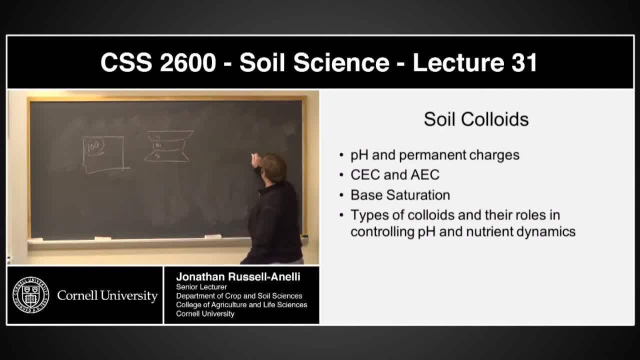 with, with, and this is when I got back to these. so if I have a silica here, you know, and oxygen and oxygen and oxygen, this is then bound to another oxygen over here, and then this is repeated structure with another silica over here. 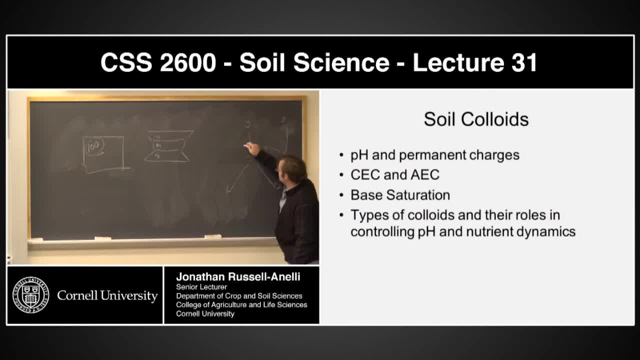 Right? Does this sound look familiar? The isomorphic substitution is the substitution of other elements in for silica or aluminum, and this is where you get the issue of the shape as well as the charge, because no element exactly the same shape or charge from silica. so if I substitute with silica, 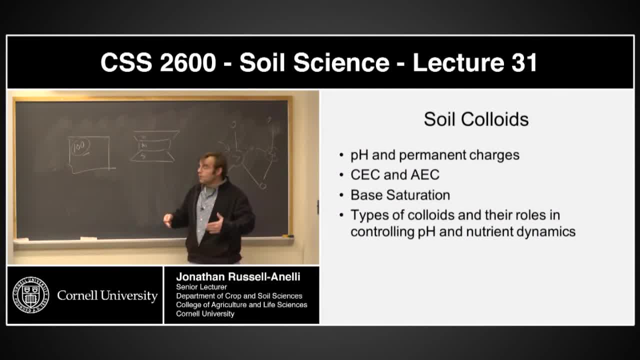 with something else. I'm either going to get the same charge or I'm going to get a different shape to my calloid. okay, that's why I showed you like the semectites have this type of shape and the kaolinites have a very flat, you know. 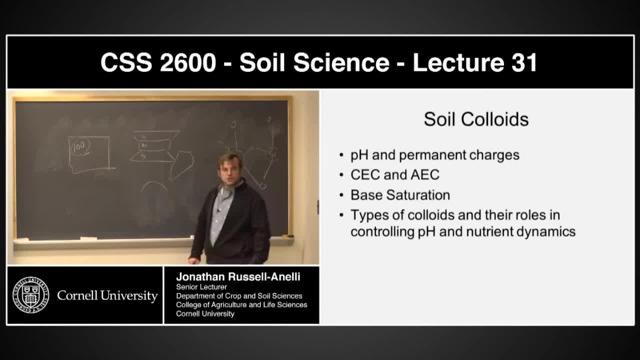 almost that kind of structure, very flat plate, like: okay, now if I put in an element, an ion, that has the same charge, I'm not going to change my cation exchange capacity from what the original structure is. but often I'm going to be putting something in that's the same size but actually has a different charge. 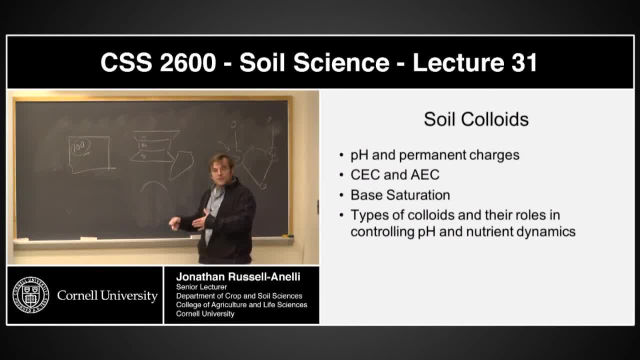 and if I start putting in one thing for another that has a different charge. say, I take an iron and put it in for the aluminum, okay, aluminum is three plus. if I put in an iron that happens to be two plus, I'm making this calloid more negative and so that isomorphic substitution in 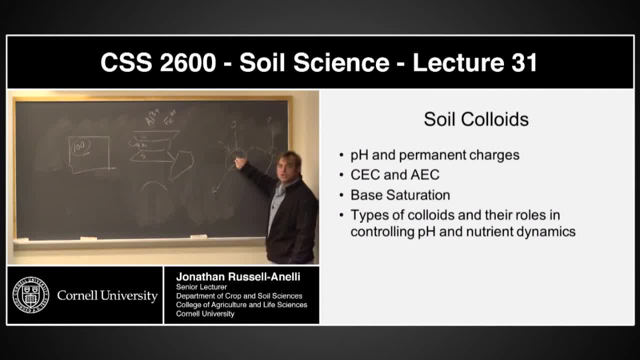 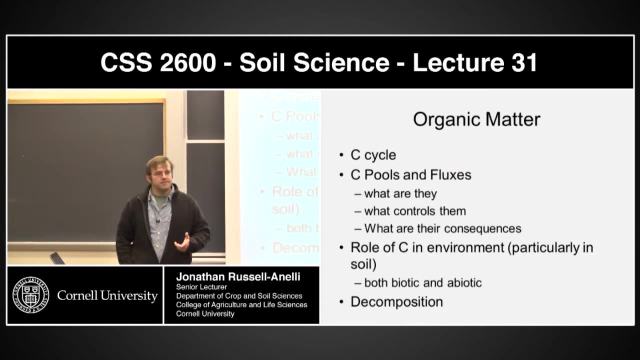 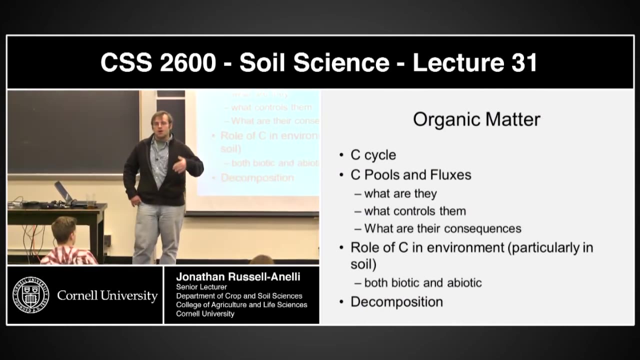 this structural, in this structure right here, is going to change the charge. ok, feel good about this one, guys, and leave this light on. can you still see this? alright? okay, so the next one was organic matter. any questions there? and we did this carbon cycle, we did the nutrient, all the nutrient cycles that were right. 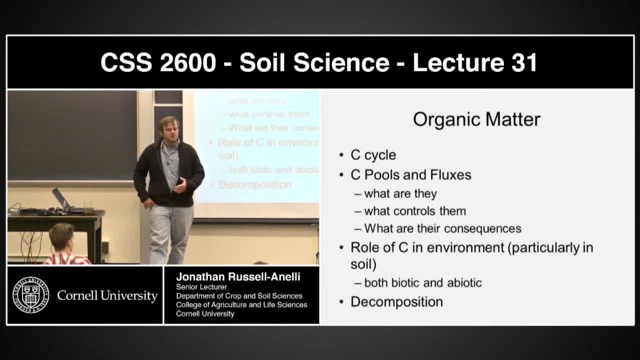 that were sort of model systems for us to think about. we felt good about the organic matter, we feel good about decomposition and CN ratios and that kind of stuff go ok. so there was a- you guys remember the CN ratio with CN ratio was it's the ratio of carbon to nitrogen, right? and there was a rule of thumb. 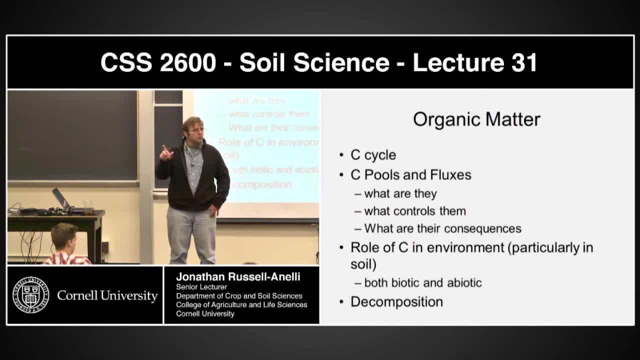 there that we said it was like 20 to 120 to one. basically is the issue it because the decomposition most of the compositions happening by microbial populations. we use the the 20 to one rule to say if it's greater than 20 to one, we're gonna have nitrogen being basically immobilized, right, because the 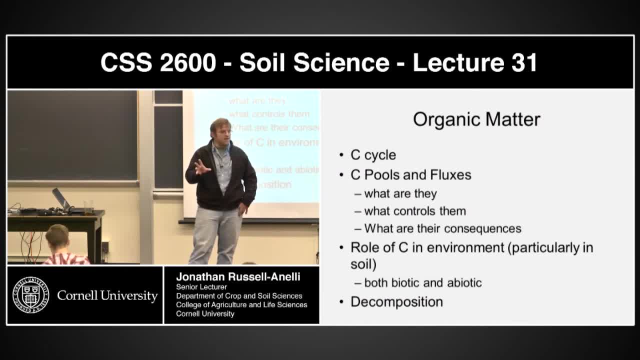 biomass issue: the organisms. the organisms have a biomass CN ratio of like 8 to 12. ok, and if you think about respiration, some of that carbon is going to be thrown off as co2. ok, if it's CN ratio is less than 20 to one, we're going to start seeing a lot of 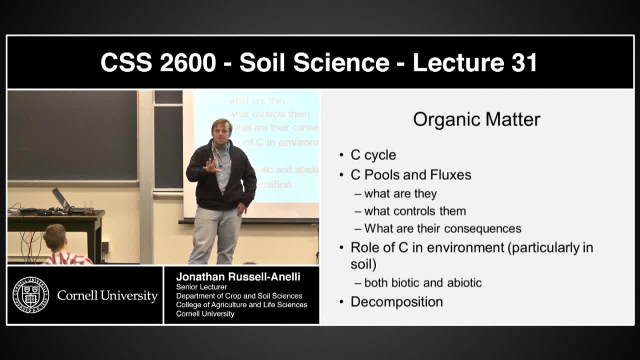 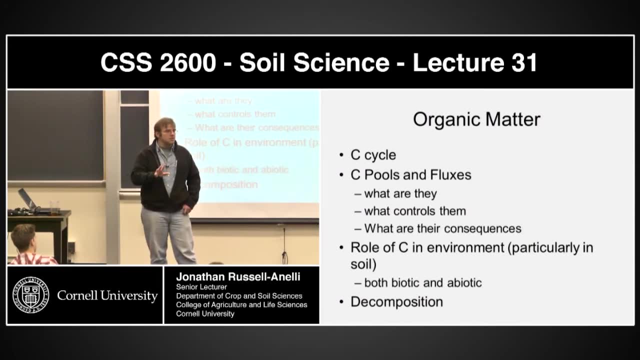 mineralization of nitrogen, because the microbial biomass they does, they don't need all of that nitrogen. does that make sense? now? we also sort of mentioned- and this is you got to take this with, take this with a sort of a grain of salt. we also said that in general, low CN ratio material decomposes faster than 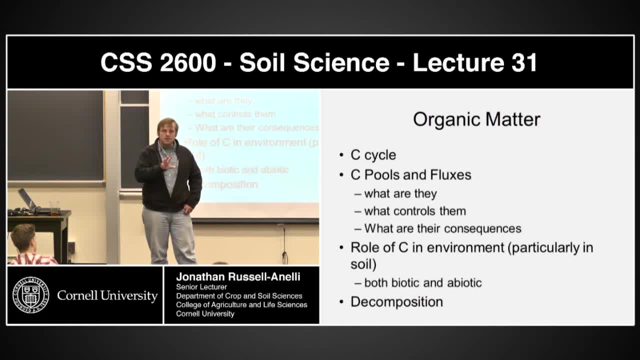 high CN ratio material, you know, but that is really dependent on this issue of what controls decomposition. do you guys remember the things that control decomposition, where there's basically four rules but the first one was the driver that really controlled everything? you guys remember what was location, location, location and that's not the 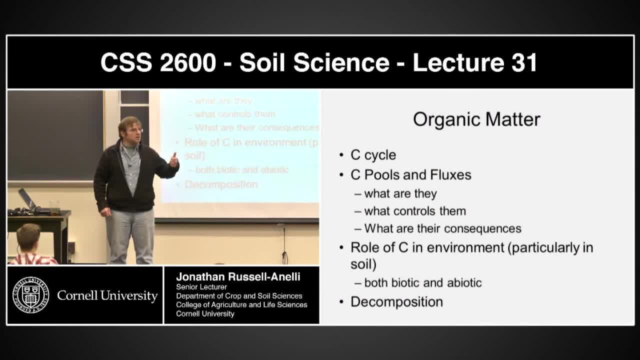 first three. that's the first one. okay, then we started talking about the quality and quantity of the material, and and then the climate that the material was in and then the availability of that material for the organisms. So those are those. Does this sound familiar? 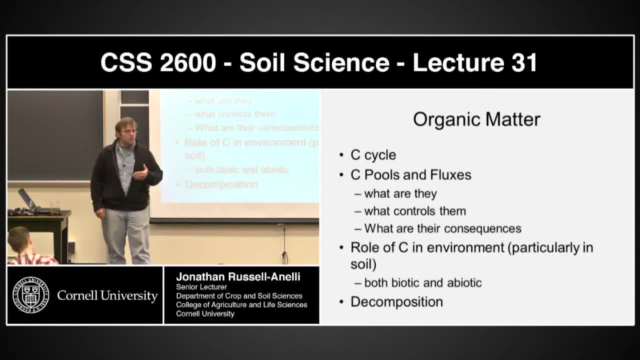 Yeah, OK, When we talk about decomposition, I really want you guys. we can talk about CN ratios, We can talk about the structural relationship of the organic molecule, And those do, are in fact, part of the drivers for decomposition. But the most important one is location. 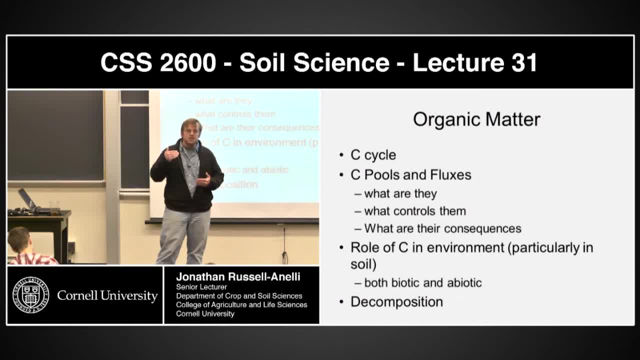 I don't care what it is. It could be sugar, It could be easy to decompose, But if there isn't an organism or the climate isn't right, it is not going to decompose. Kata, and then we'll go. 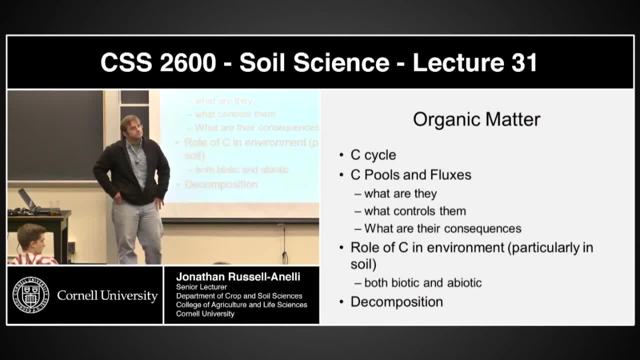 Go ahead, Doesn't Kata go? So you talk about location and climate being very difficult And I'm just wondering: where does an issue come from in aeration? So location can mean a lot of things. Location can be- I mean you, literally. 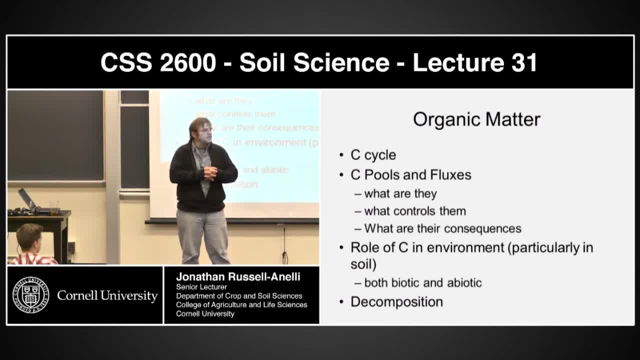 can have an organic molecule being occluded. It's covered by something and the organisms can't get to it. But you can also have an organic molecule located in this prime location, except there might not be any organisms there Now. you also could have an this. 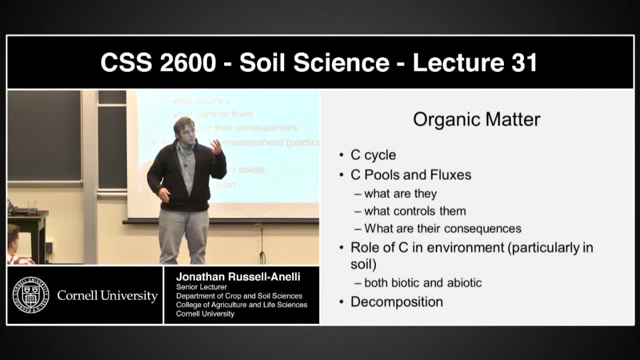 is where location sort of trumps everything else. If that piece of material that's going to be decomposed, or potentially can be decomposed, is in an area that's warm enough but not wet enough. that's a climate control, but it has to do with location. 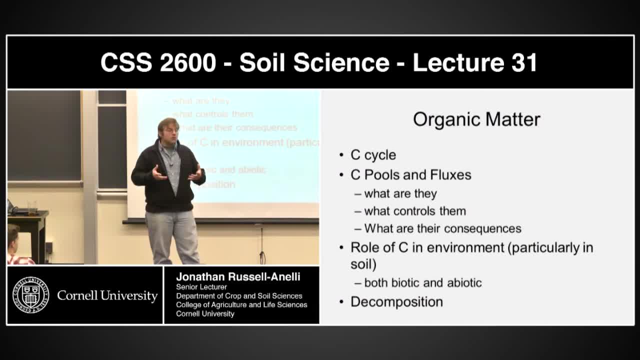 So they're interacting there. Now this also gets into this issue about where the organic matter is put into the system Around here, most of the organic matter that's put into the system comes in at the surface because we have leaf, fall and things like that. 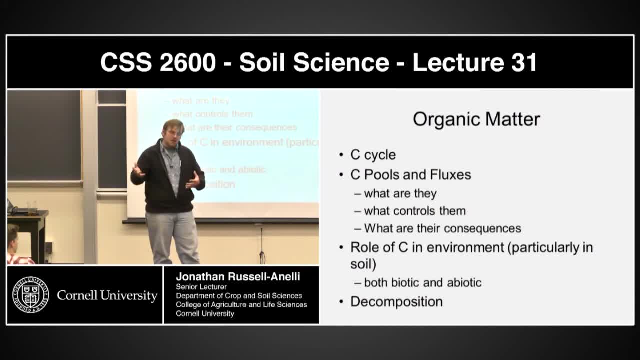 But you start moving into mole soils, grassland systems. yes, there's some coming in from the top, But a lot of that stuff is way down below. And then you have to start thinking: well, the organisms that are doing the decomposition. 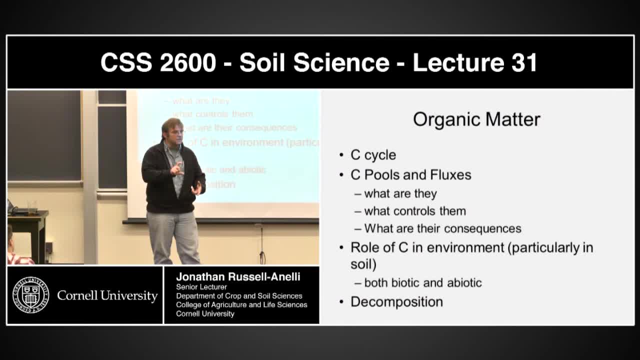 they have a very select part of the environment that they live in. Now, do you guys remember me talking about the actinomycetes? This is a really good example. Actinomycetes were those spore-forming sort of filamentous microorganisms. 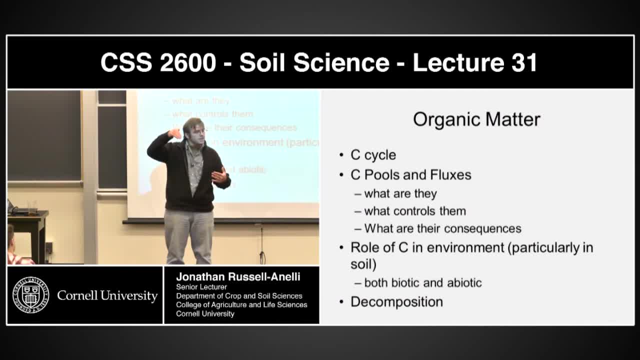 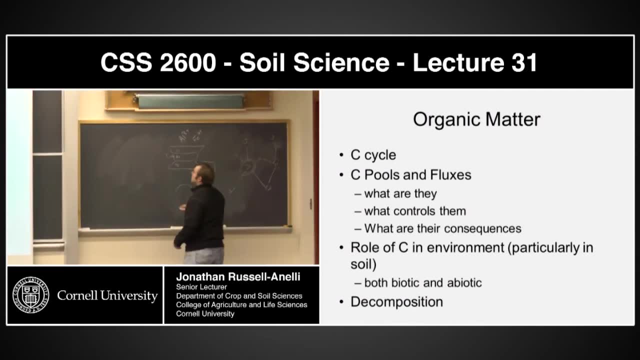 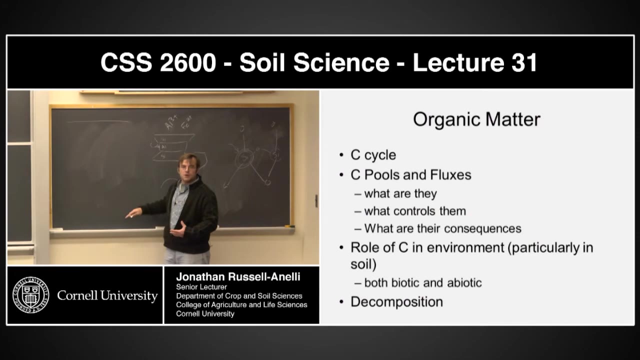 And they basically sort of make colonies And those colonies can bridge And they can make different ecotypes or ecotones inside the soil system. because here here's my soil surface, As I go down through the soil surface from the top to depth. 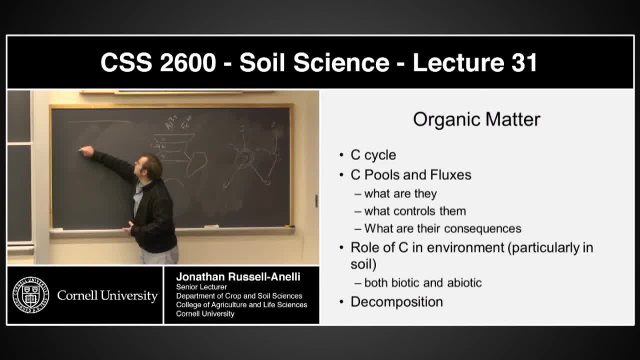 where should I see most of my organic matter Up here? So this is why we have O's and A's up here. But this system is also very variable climate-wise. It starts to get sunny outside. That means this is going to get dry and hot. 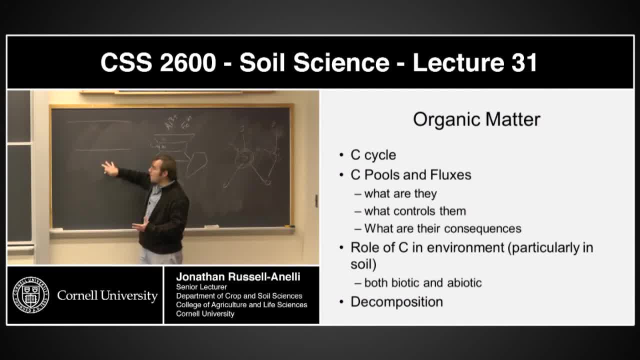 It rains, It's going to get wet and cold. Farther down, climate is more constant And it's not amazing. but water flows downhill, So in all likelihood this is going to be moisture. So I have an organism that up here. 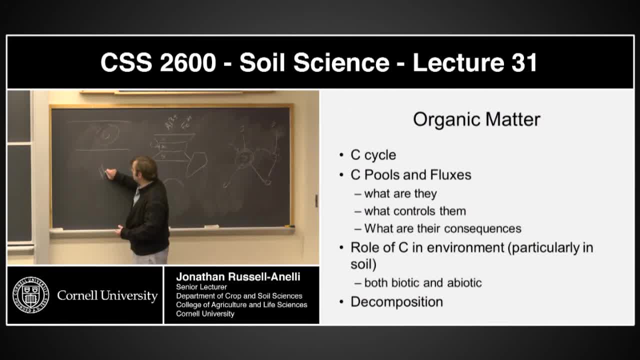 is where my carbon stock is Down. here is where my moisture is. Now, if it's dry up here, this carbon stock, nothing's going to happen to it. Now it may be wet down here, but if there isn't any carbon stock, 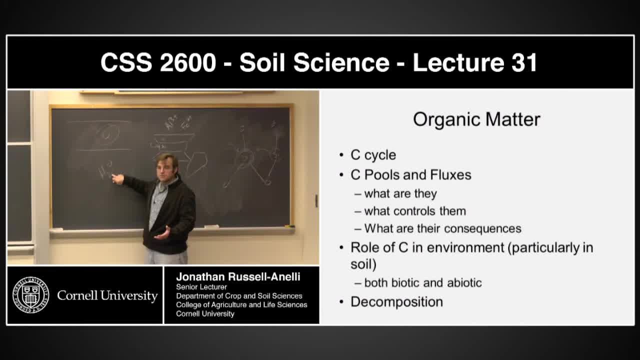 down here it's not going to get decomposed right. So these actinomycetes basically can build colonies that bridge this divide. So, in essence, the organisms are. forget about the actinomycetes, Think about earthworms. 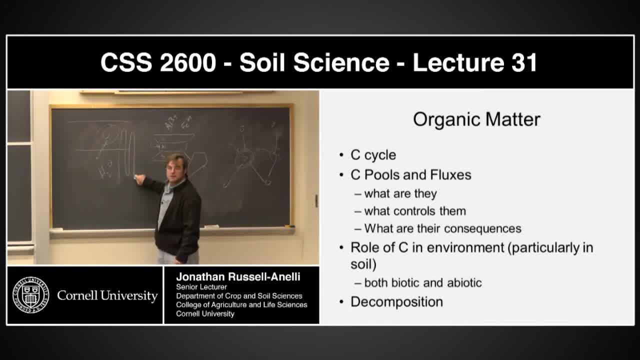 Earthworms, because of their motility, can do this. They go up, They grab the organic matter, They go down shelter. So basically earthworms overcome the limitation of location because they have motility. But if I have a microbial population, 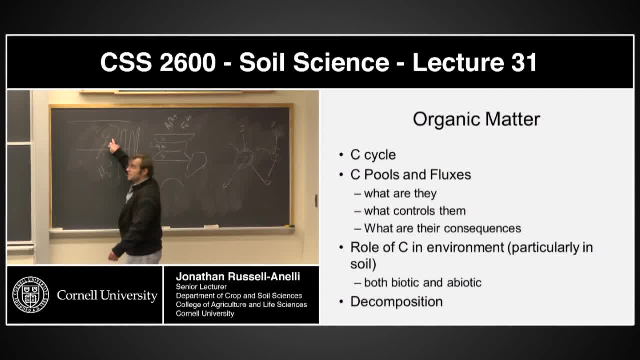 one Pseudomonas sitting here. if he's not near where that carbon is, he's basically out of luck. Does that make sense? So the location of this carbon has a huge impact on its decomposition? Does that answer the question, Kata? 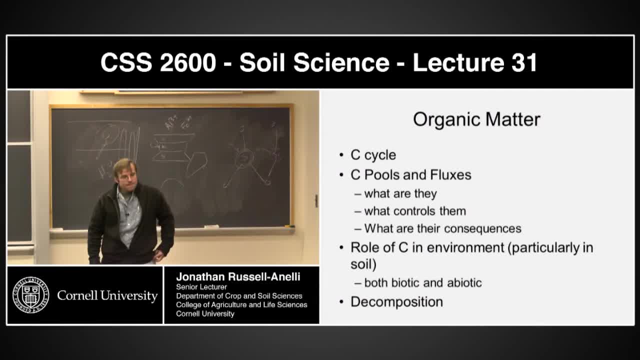 We'll hold off on that one for a bit. Madeline, you had a question: The difference between location and availability. The difference between location and availability Availability has to do well. first off, obviously it has something to do with it being there. 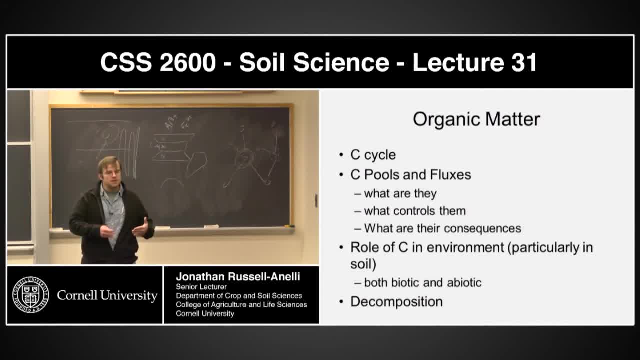 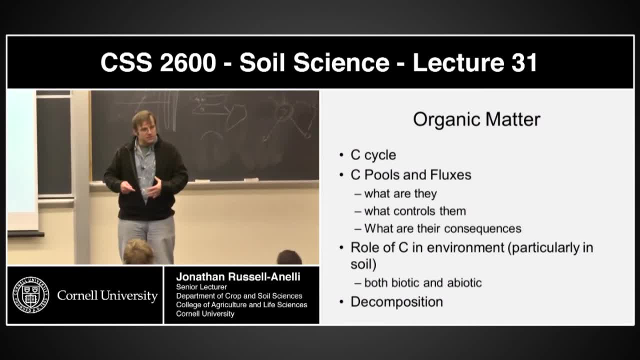 But it also has to do with the nature of that material. If I'm an organism, that, if it's a wood chip or something like that and it's me, I can't eat, that I don't have the biological system that can decompose that. 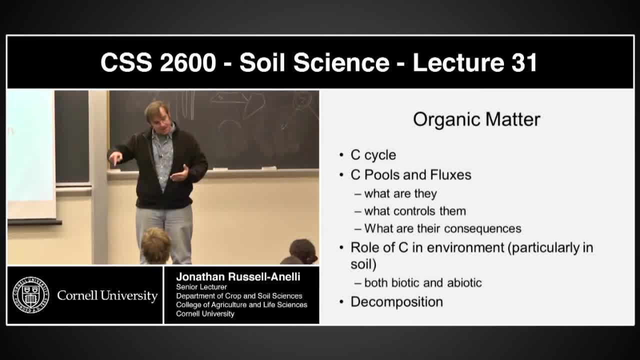 So you have to have a specific organism that can, in fact, attack that piece of organic matter to decompose it. But isn't that quality? That's quality. But see all of these things, they're all interacting into each other. 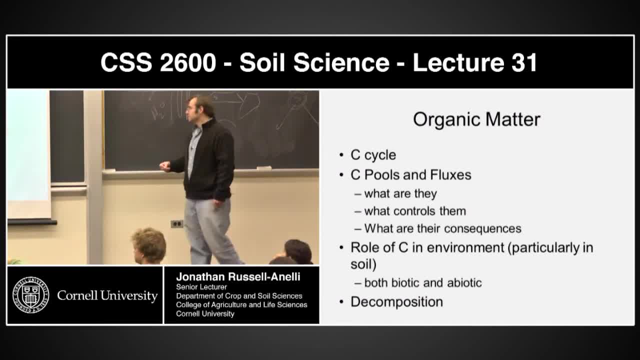 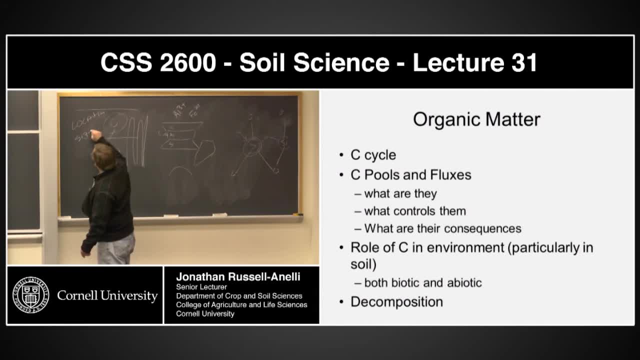 The four things that you have in the notes are slightly different than the four that you mentioned. OK, So the ones in the notes are placement, size of the area, the N ratio and litter quality. So the microbial population and the climate all seem to be locked into the location. 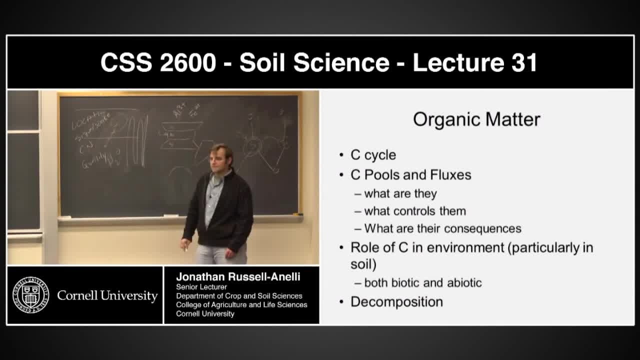 And the availability piece is part of the quality, But the one you mentioned a minute ago, there was location, there was climate, which may be part of our confusion. that- And there's quality. So what you meant. so that's what's in the notes. 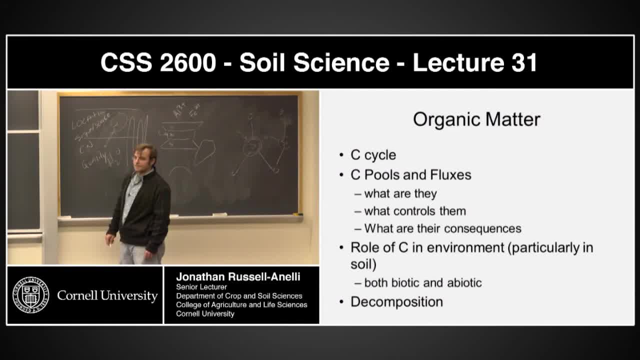 And then the four you mentioned a minute ago were location, quality, climate and availability. But in the notes it seems like climate was part of was locked into location, which may be why we're confused as to how location Availability 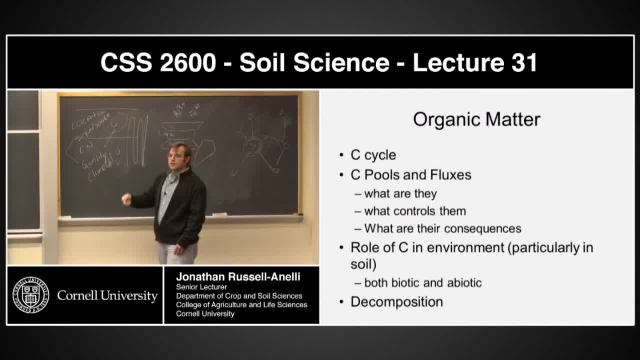 Yeah, Interact. OK. So the notes are saying location, size and surface area, CN ratio and quality. OK, So back to location. When we talk about location, in essence we're talking about an issue of quality as well as sort of the size and surface area. 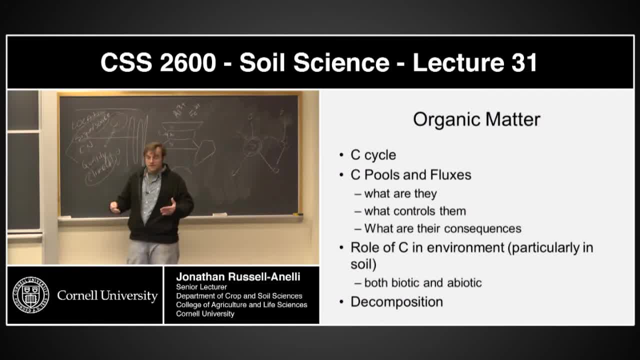 OK, Because if it's being deposited on the surface, it's probably larger material As it starts being decomposed. and this goes back to that net bag, that mesh bag experiment that we looked at. you know, location is going to have a lot. 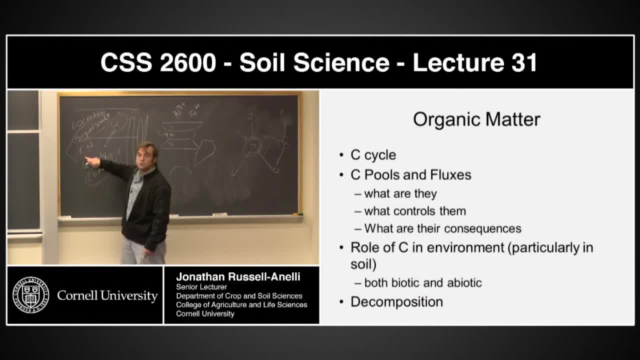 or size and surface area is going to have a lot to do with what has happened to it, Right, OK, And now back to this issue of availability. that relates to all three of these. Actually, it relates to the location one as well. 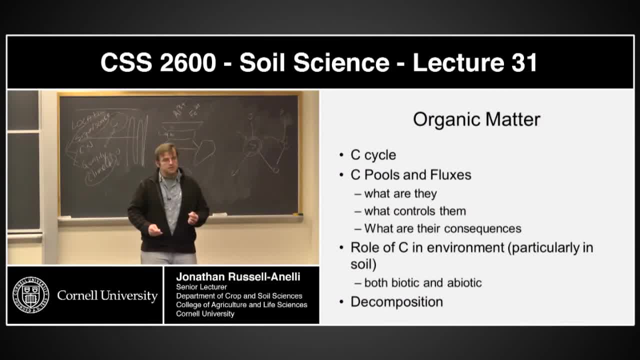 But availability of a material is not just: do I have access to it. Availability of material is: can I in fact react with it? OK, And that is this issue of CN quality as well as, in a sense, climate. 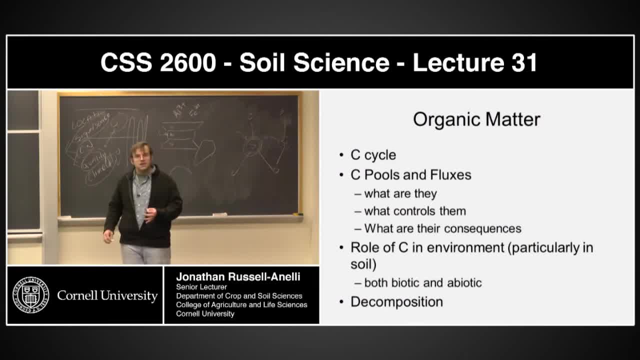 OK, So these things are controlling that decomposition, But it all comes back to this one, because this one basically, to a certain extent controls all of these. It doesn't really control the quality per se, other than the processing issue. 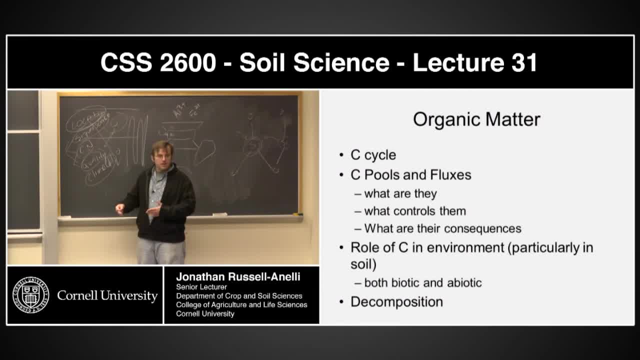 OK. So if it's gone through a worm's gut, the quality has been changed. OK. If it's gone through a worm's gut, it has a lot to do with location. OK, That worm is going to be pushing the pieces out. 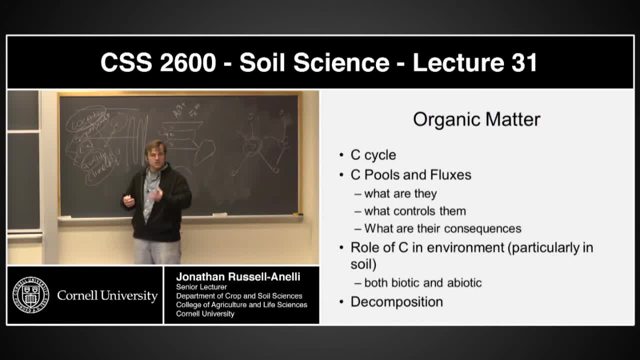 at very specific locations. OK, basically through the worm tunnel and in the casts. OK, Did that answer the question? That was a common question. yeah, sort of Go. So it seems pretty clear by that, like what the biotic? 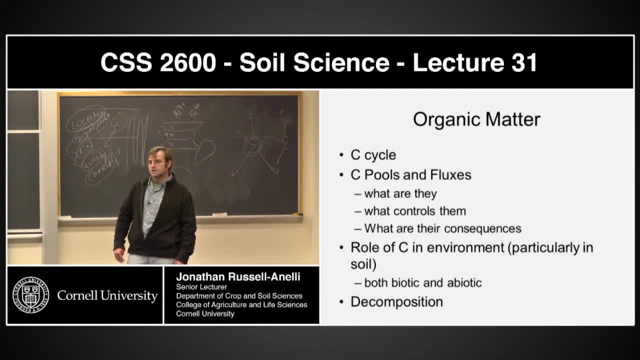 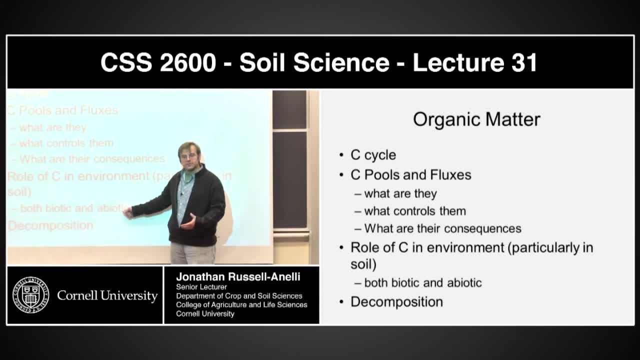 what's the role of carbon in the biotic here and what's the abiotic? The abiotic issue was: what do these things potentially do, What do the products potentially do? And we did this in the lab when we looked at the corn. 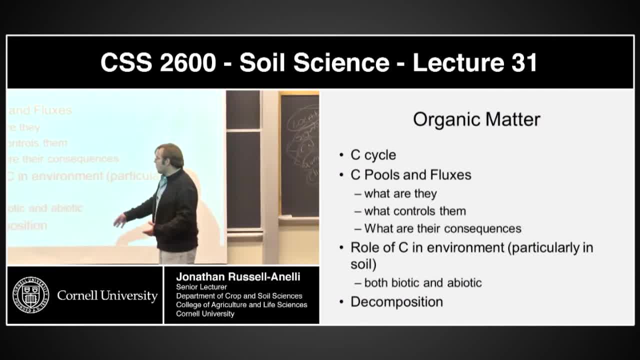 the cucumber seedlings. OK, There is this sort of hormonal response from this organic material. That's one That's in a sense that biotic. But we also talked about these guys' role on the climate Organic matter. well, you got. 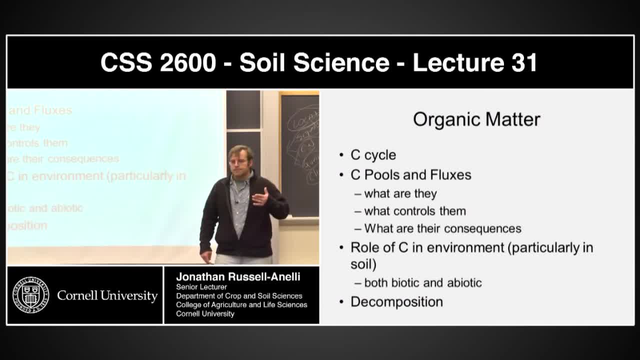 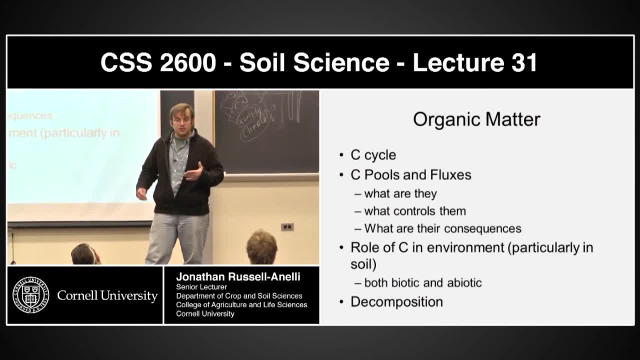 not all of you have done this yet. OK, From a climate perspective, what does organic matter do? If I have more organic matter in my cells, I'm certainly imagining that I'm going to have more water storage because of the sponge effect. 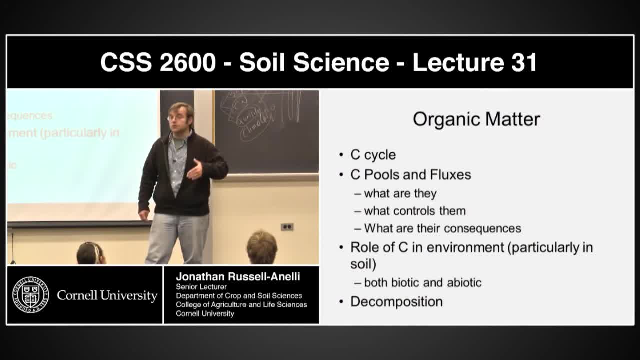 Potentially, how it's distributed is going to have a huge impact on infiltration. OK, But this is also going to have a huge impact. organic materials also going to have a huge role on temperature. Right, If I have a black surface and I start shining a light on it, 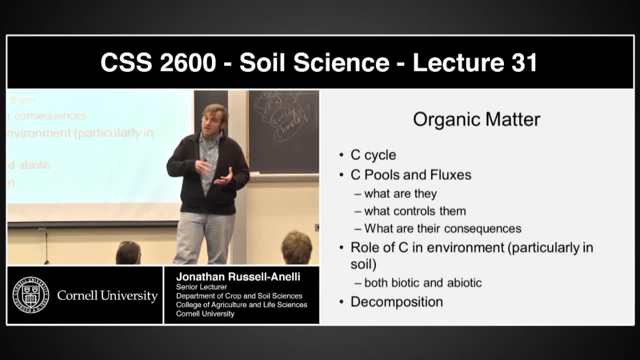 it's going to get dark, it's going to get hot, But on the other hand, these tend to have low bulk densities and because of that bulk density, the transfer of that heat is going to be very different. And this is when we start talking about mulch. 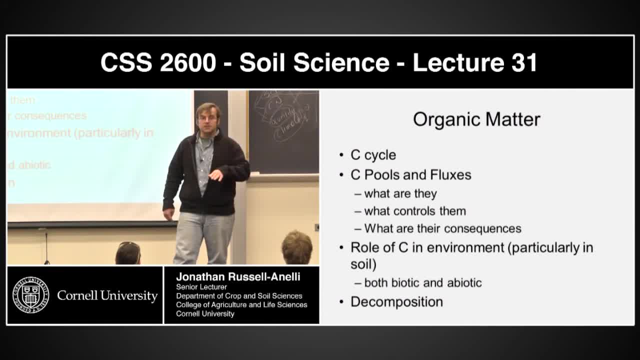 Those of you who have been in lab this week already have an understanding that if I put a heat lamp over a black material- organic material- it's going to get hotter than a lighter material, But that transfer of heat is not going to be very far. 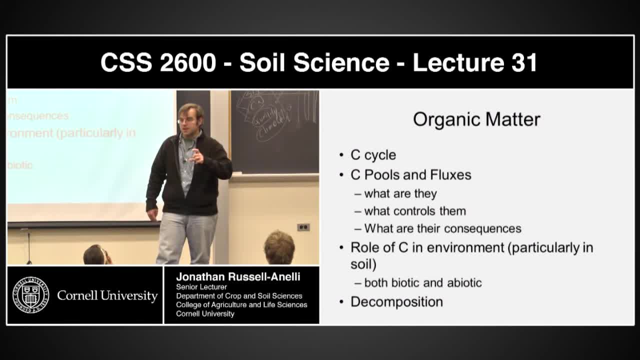 because of the porosity or the void space of the, the organic material. It doesn't take a lot to heat up temperature, heat up air, but air doesn't have a lot of energy to transfer that heat to other things. OK, So abiotic controls. 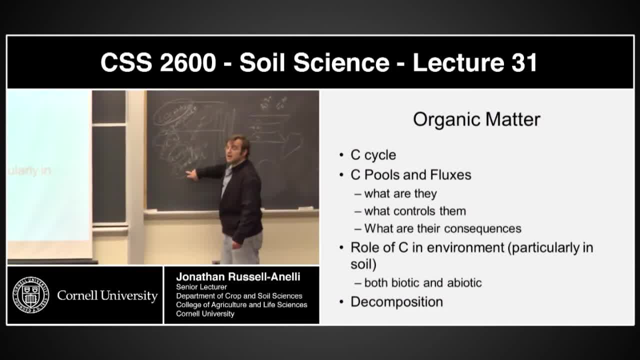 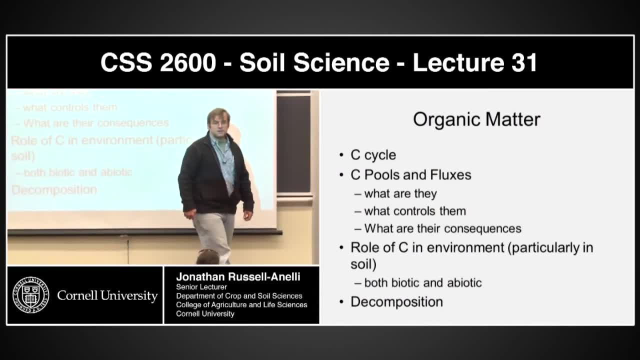 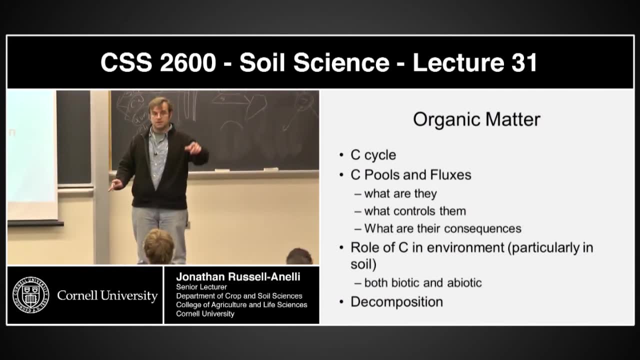 have a huge effect on this issue of climate, which, in turn, will have a huge control on decomposition. Yes, No Kind of Good Go. How much do you want us to know about the composting process? The composting, oh, composting process, yeah. 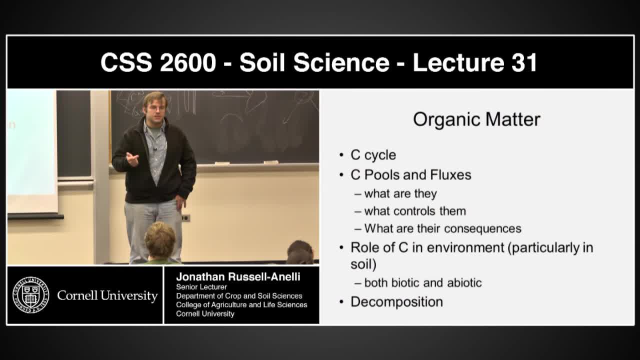 I want you to know about it. I want you to have an understanding of actually more importantly than the composting. I want you to have an understanding of how this is more soil ecology than organic matter. but I want you to have an understanding about 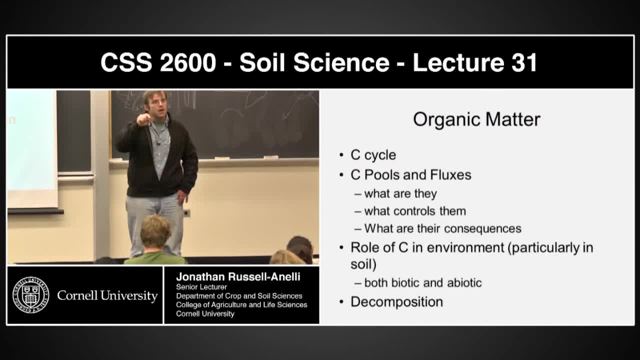 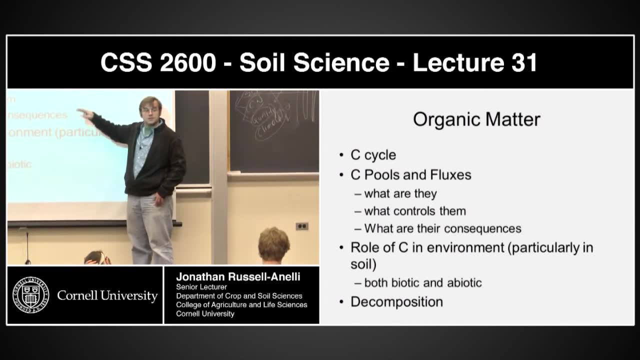 the feedstock and its response and the response of the population, the ecological population, that are interacting with it. And then what are the consequences of that on the environment, And not just on the environment but on other organisms? Do we feel good about this one? 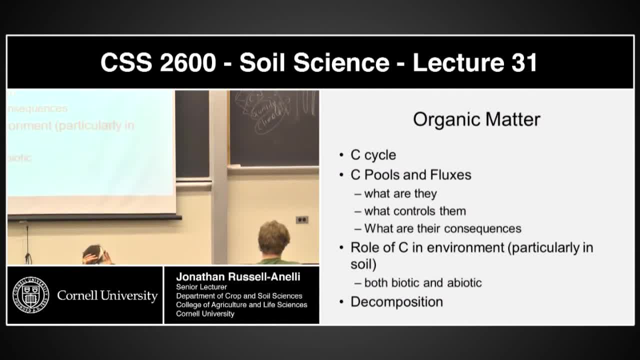 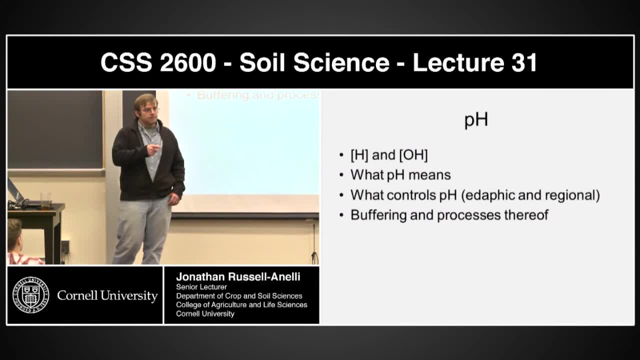 Can we move on to the next Ph? Can you give a brief overview of the gas that you use? And this: oh, what controls PH? locally and regional, regionally, Okay, so when we're talking about, let's start with regional. 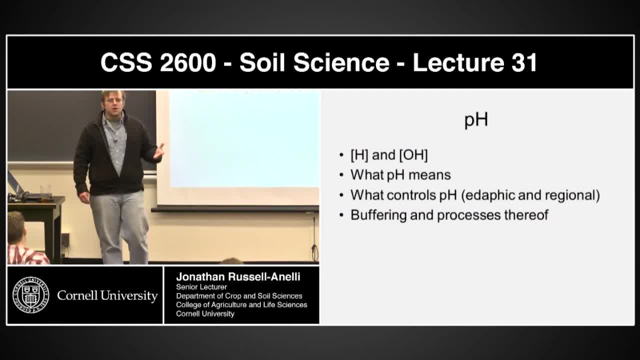 because that's, I think, that one might be a little bit easier to. so what are the controls on PH, regional sort of PH issues? The obvious and first one that we should all be thinking about is what happens when it rains. Okay, rain moves through the system. 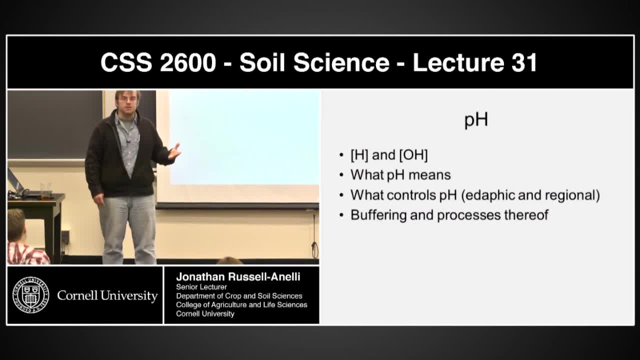 the air? okay, the air has concentrations of CO2 in it. what is it going to make? Carbonic acid: okay, this goes back to the weak acid. in a million years it can weather everything away, but you know. 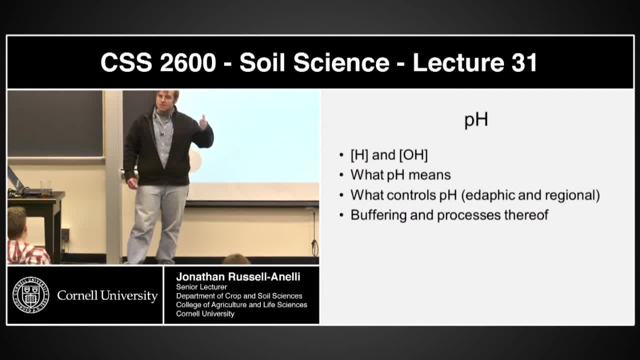 every time it rains. now there may be other things coming in with the moisture, but every time it rains, I'm going to be increasing the proton concentration of my soil solution. okay, and the consequences thereof, which we've already talked about. 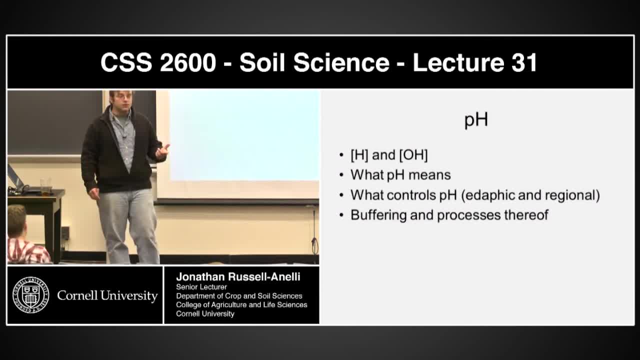 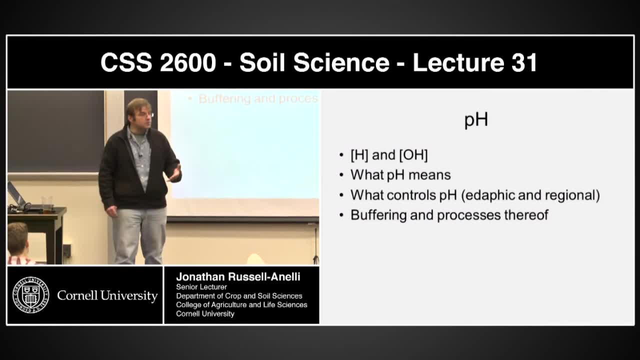 okay. Now there are other sources of acidity that come in from regional sources- okay. these could be natural sources, such as a volcanic eruption, okay. or and the rain water, but it also could be anthropogenic sources, such as acid rain. 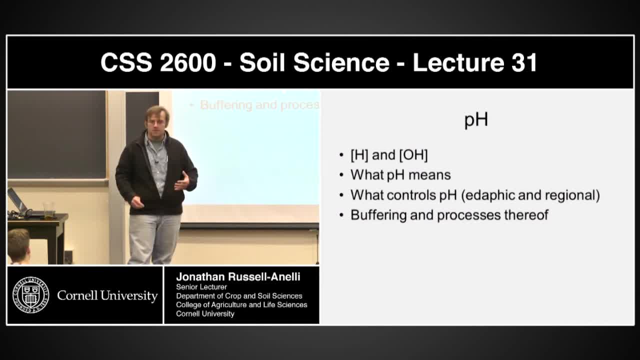 okay, coming from stack emissions, from emissions from anything that's pushing out NOx or SOx up into the atmosphere, That NOx and SOx is going to interact with the water and it's going to make nitric acid or sulfuric acid. 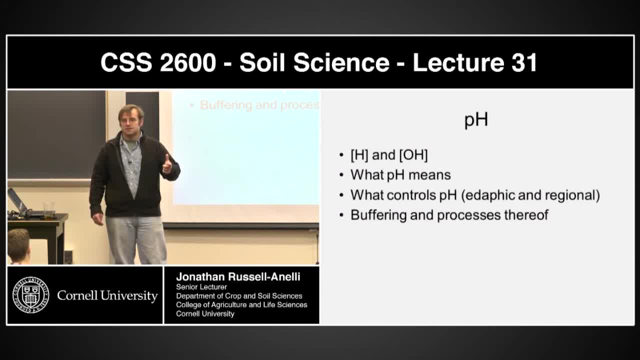 okay, these are strong acids. They hit the ground and they're going to acidify the environment that they're in. They may not make it acidic, but they're certainly going to be linked to the environment that they're in. So what are the local controls? 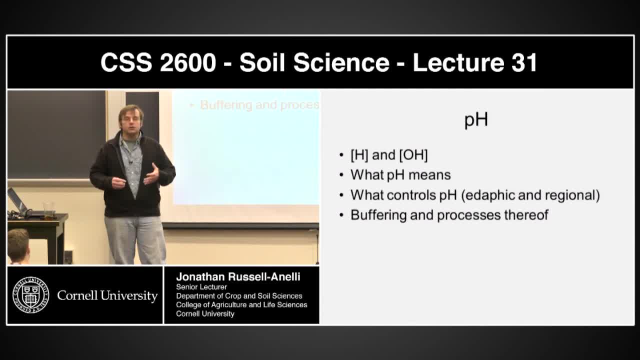 for lowering the pH. Those are regional controls right Now. what are the local controls on pH? Certainly, as the parent material. the first one is really parent material. The second one is biological activity. Okay, parent material as it weathers. 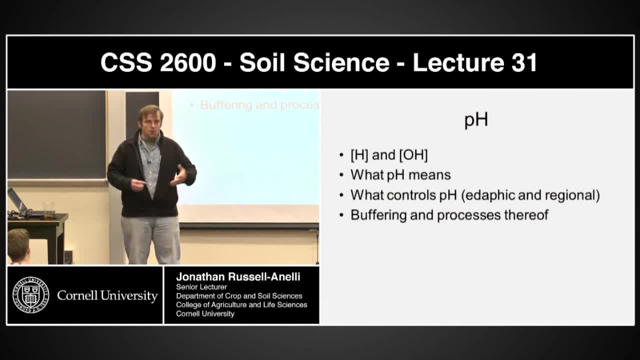 it's going to be throwing things into the soil solution. okay, A lot of those are going to be bases, so that weathering, in a sense, is going to be acting as a buffering. okay, But weathering of pH or weathering 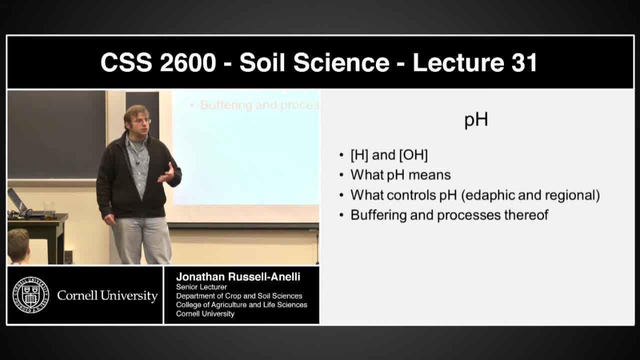 of primary minerals or secondary minerals, of rock material is a slow process, But biological activity, on the other hand, is really fast. okay, Generally, biological activity produces acidity. okay, Decomposition processes produce acidity. Now, those that acidity. 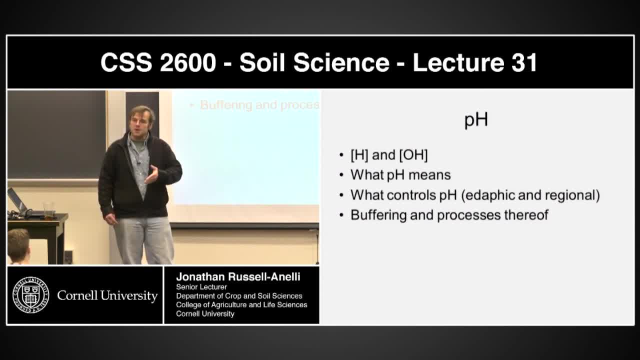 is going to be localized to those organisms and it's also going to be dependent upon material to actually decompose. Does this sound familiar? Go So, adaptive would just be local. Local. So if you have a situation where there's runoff, 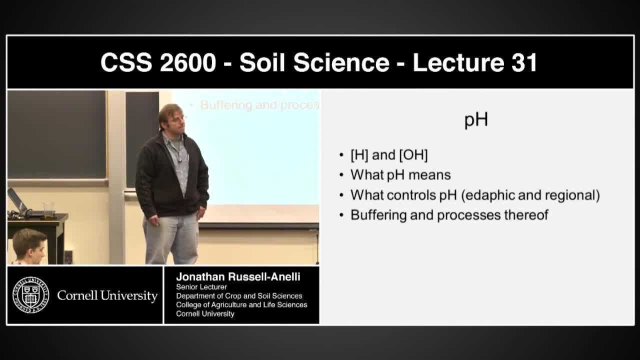 from sewage. would that that would be adaptive? Yeah, I mean we can talk about the specifics of that. I mean, if it's, if I have a. so the question is if I have a, a source of sewage water. 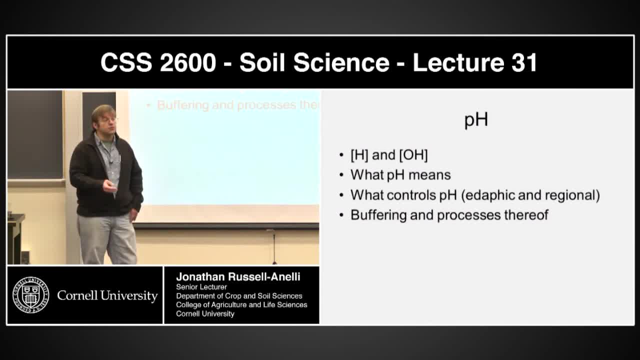 or something like that. I mean you can certainly imagine acid, mine waste and stuff like that coming out in the streams. Is that considered reasonable or adaptive, or local? Yeah, I think it's a scale dependent thing, I would. I mean. 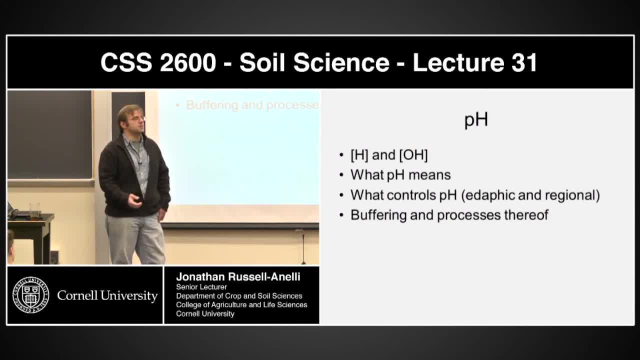 certainly I would imagine the sewer system being a sewer spill or something coming from a septic system or something like that. I would think of that as a local effect, But it's certainly there are downstream effects, I mean you can think of. 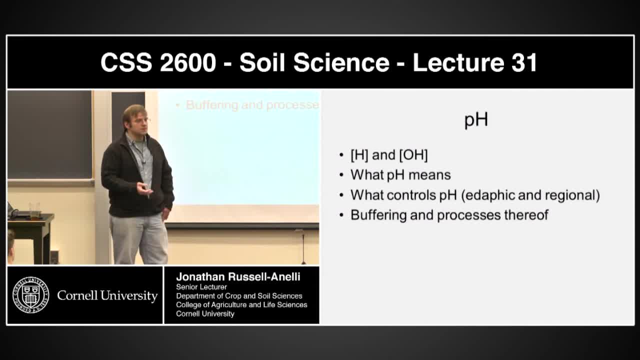 manure applications and stuff like that. Yes, there's a local effect, but there's also a regional effect. Are there any processes that raise the pH, aside from the like you mentioned, the buffering and stuff? Well, the weathering of material is actually going. 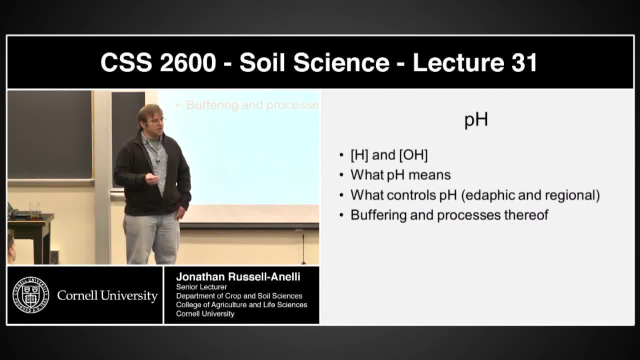 to raise the pH. Okay, Are there any short-term things? Short-term raising a pH? not really Most. most biological activities, most sort of, unless unless it's an abiotic process that's a result of acidity or something like that. 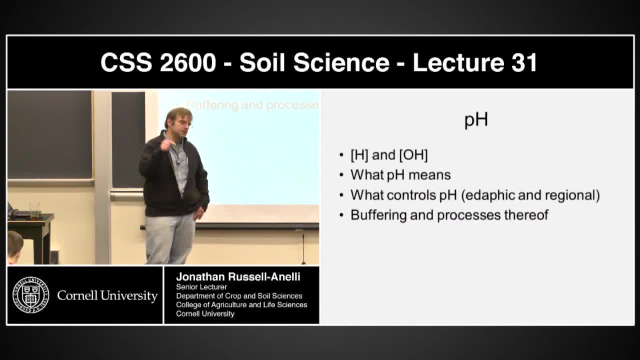 driving weathering processes, Most of the system. we are always sort of driving towards acidic systems. Okay, But then so rain comes and then it dries out. does that raise the pH, Like rain comes and then, Oh, sort of a fluctuation? 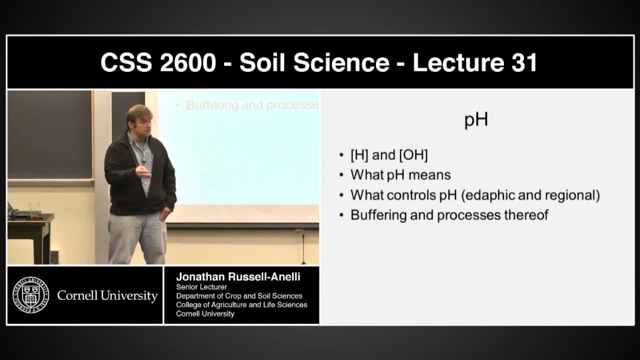 type of event. Well, yeah, certainly you can have situations like out west where you're looking at rain systems that you know this is sort of more salinization, but the salinization is going to raise the pH, So I have a rain system. 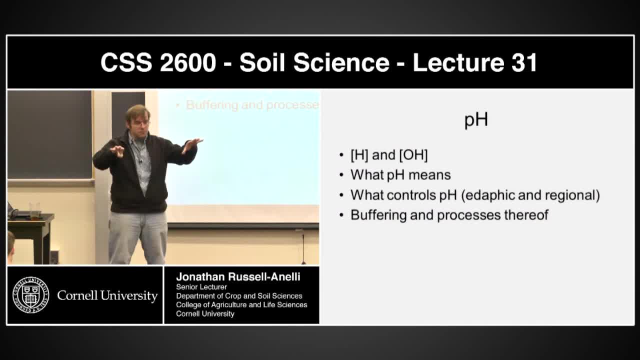 water hits the entire system. it solubilizes stuff. it was soluble. the water basically moves down into the bottom of the basin. okay with the soluble salts. When the water starts evaporating and the salts are left behind, that's going to be. 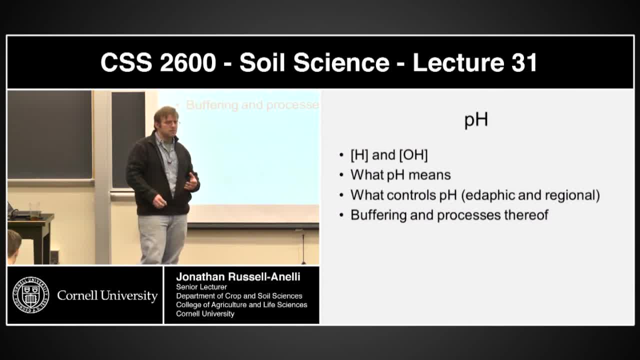 raising the pH. Is that the type of situation you're talking about? Well, we've been thinking like. here we have a rain event, something some area saturates, Right. It becomes more acidic once it, you know, a few days later. 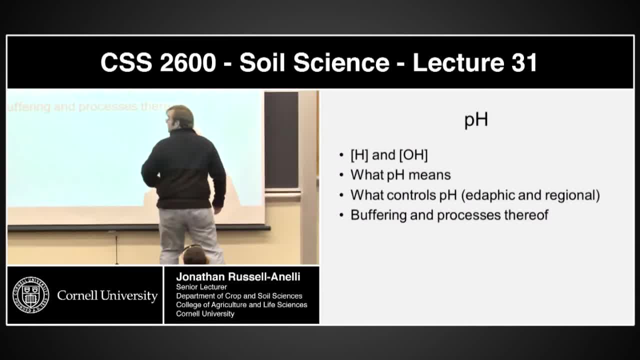 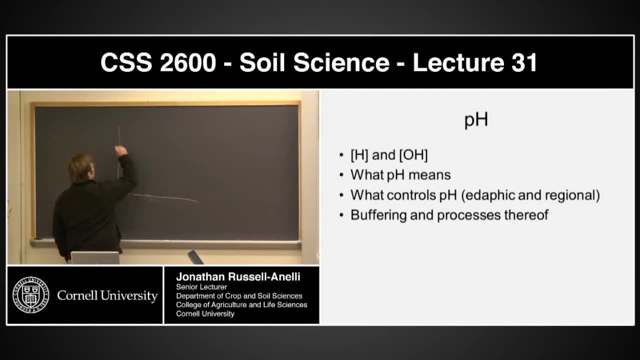 once it drains. Yeah, so, yeah. so I mean that type of scenario which you're looking at. I think you're looking at something, a scenario that's like this, where we have wetting and drying sequences, and this is time. 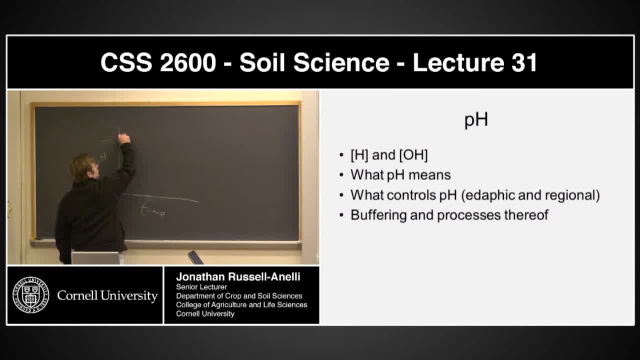 You certainly are going to see. you know, generally, the trend that we're going to see is something that looks like that. okay, but the reality is that it's going to be doing that kind of stuff to get down there. okay, Does that make sense? 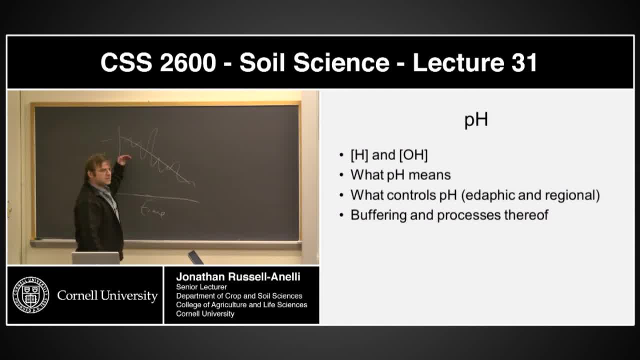 to everybody this issue? Okay, it's not like it's, you know, and there's certainly geologic processes and things like that. So you're really talking about sort of a time scale. What time scale are you talking about? 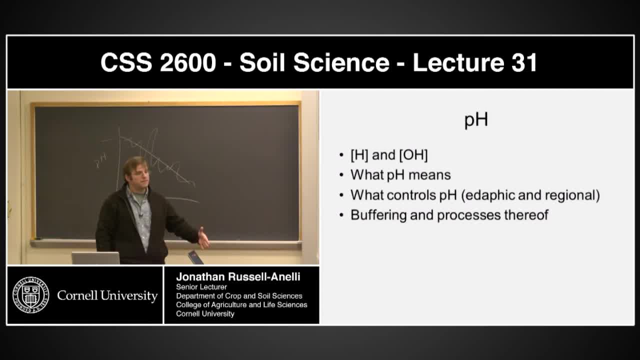 Are you talking about an ecological time scale? Are you talking about a geological time scale? You know, if you're looking at an ecological and pedological time scale, this is what you're seeing: Pedological soil. okay, When you start looking. 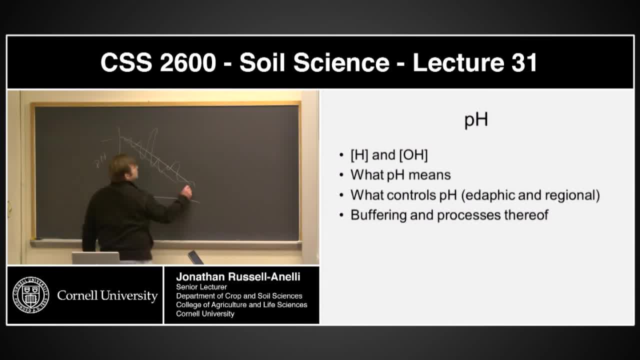 at geologic time scale. this is not necessarily. I mean you could be seeing this and then all of a sudden you can have some sort of event and you know it's. I mean all these stochastic events and even in the pedological 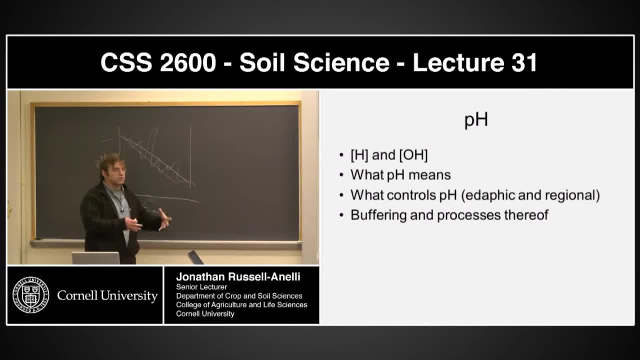 I mean, you can have a stochastic storm coming in bringing material, but in those types of systems you're starting to see regional effects rather than a data effects. This is what you're going to be seeing. okay, This is not until you sort of see. 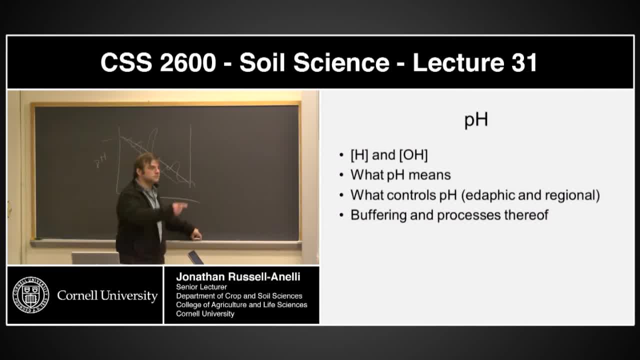 some sort of regional stochastic event? Is there a correlation between CN ratios and pH? Well, I mean that off the top of my head. I don't have a clear answer on that one. I think to tend to think that as the CN ratios decrease, 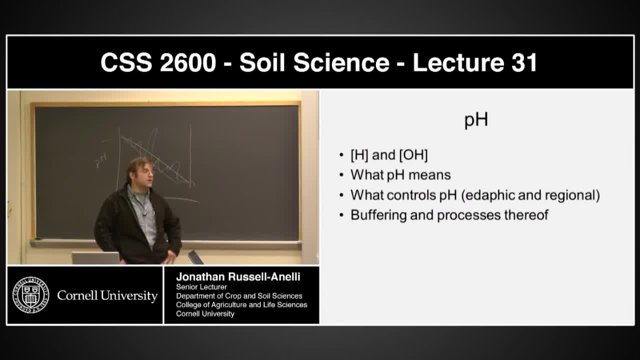 we're seeing, in general, more rapid decomposition and if we have more rapid decomposition, we're seeing more biological activity, which would create more rapid acidification. But I'm not sure that that's a trend that we should. yeah, I'm not sure. 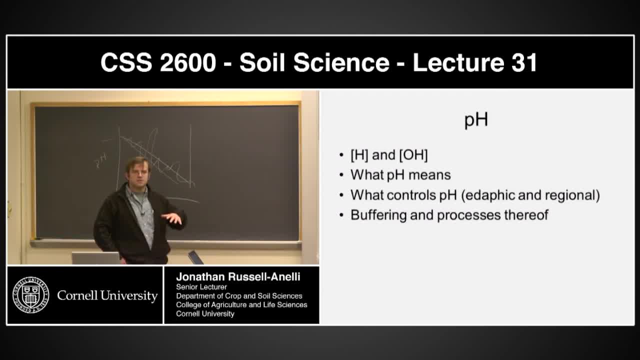 that's a strong correlation. So any other questions on this one Hold on go. So with more rapid decomposition, more biological activity, We expect the pH to go down right, Right, Become more acidic. Now how does that explain? 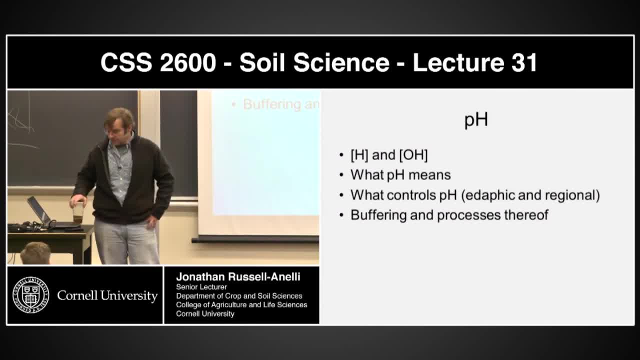 in, like the pHs we saw at the compost that were actually, Ah, that's a stock material, Okay, So the compost is a really good example. Okay, Generally, when we think of decomposition, you're seeing, you're thinking, I'm seeing acidification. 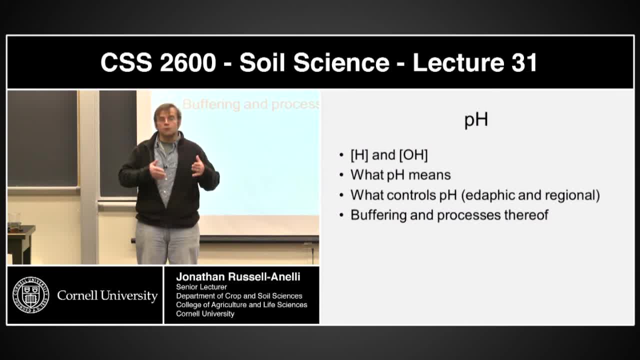 But acidification is not necessarily a measurement of pH. Acidification is a relative measure of pH. If my material ends at 10 and it ends at 9,, my pH, these are still alkaline materials, but I am seeing acidification. 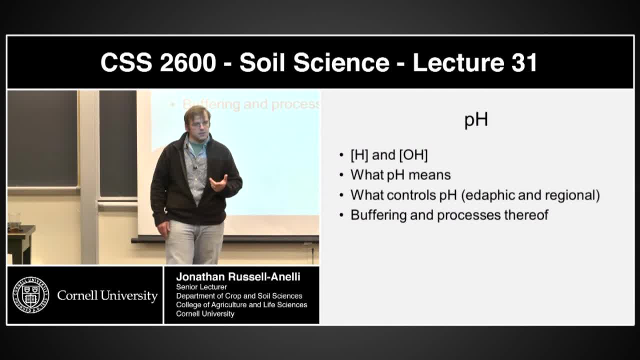 Now, part of what we're going on with the at the compost facility is this issue, that of our stock material, Where, what is the material that we are decomposing? Yeah, Okay, And you got to think about where it comes from. 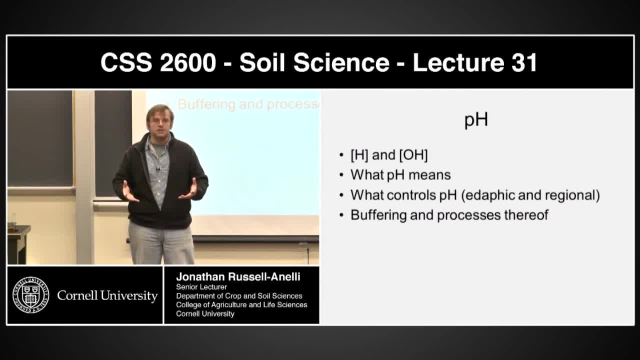 Well, if it comes from cafeterias, you know there's a lot of salts in it. We just put salts in our food, probably too much. Okay If it's coming from barn waste or something like that and scraping up the cement pad. 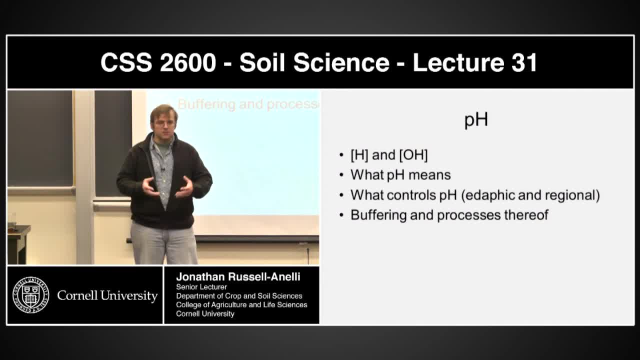 you know you're going to be picking up calcium carbonate from the limestone that's in the cement that's going to be out there. Okay, And so, as a result, we- the compost that we have- tends to have a lot of salts in it. 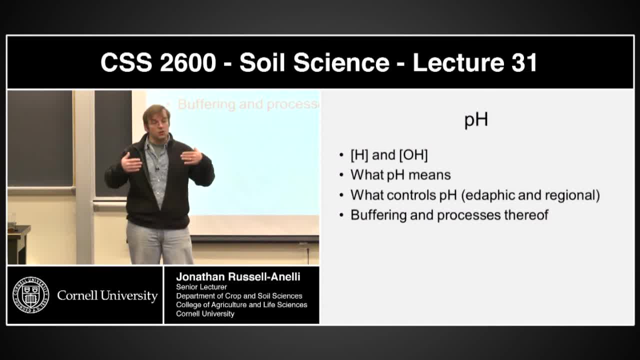 And that's why it goes through that curing phase where actually not the curing phase, where it goes through the rinsing phase, It's not- we don't call it rinsing phase, but it's basically rinsing. That's why it sits. 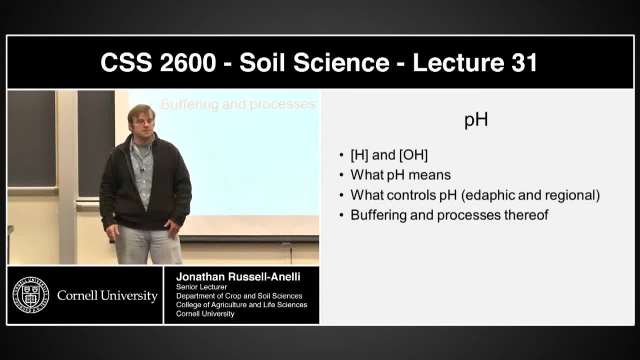 in that big windrow and it's exposed to the real world. for, okay, All right, let's move on. Oh, Madeline, you had a question. Just like the buffering of calcium carbonate, Uh-huh, So the calcium carbonate? 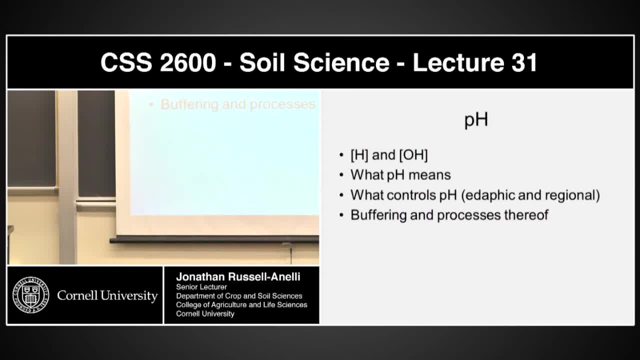 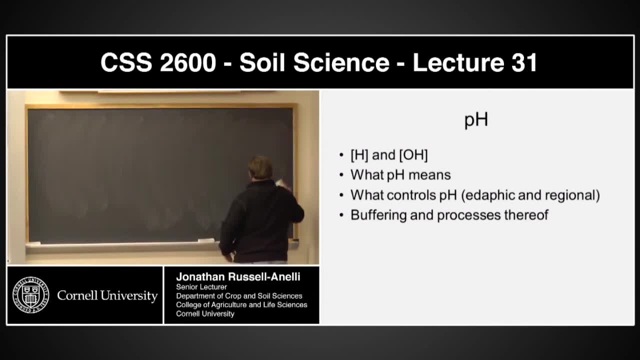 buffering reaction. This is the buffering at the high end. So let's, you guys did an experiment in the lab And you did. basically, you used two buffering reactions of calcium. One was a calcium hydroxide. This is one you started with. 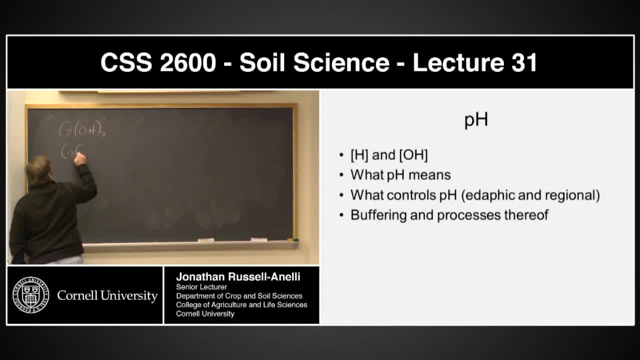 And the next one was calcium carbonate. That's an A, Sorry. Okay, Now we add an acid to this. What's going to happen? Well, you start adding the acid to this And we'll make this as a balanced equation. 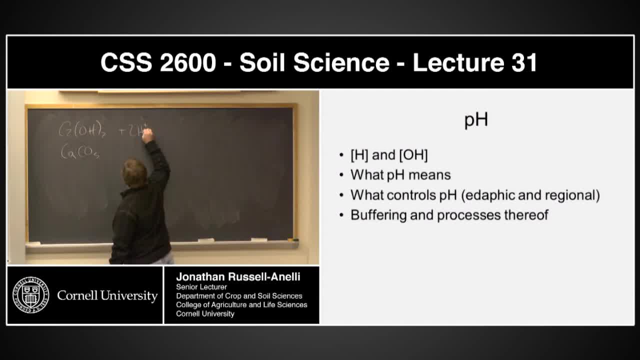 Okay, Two protons. They're going to react with that hydroxide, Okay, And basically, what they're going to do is they're going to. basically, what they're going to do is they're going to put calcium into solution. 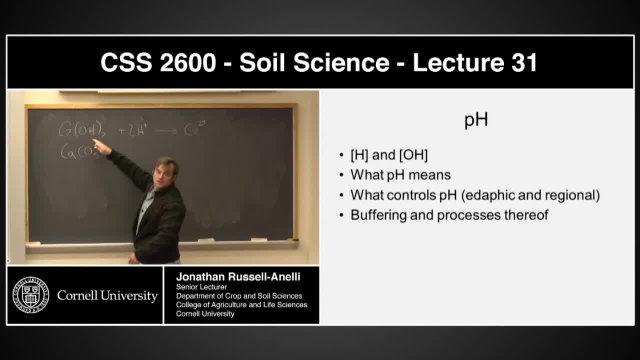 This whole system is an aqueous solution. Right, It's not calcium hydroxide powder. Okay, I add the acid. These protons are going to react with that hydroxide And it's going to make water. It's actually going. 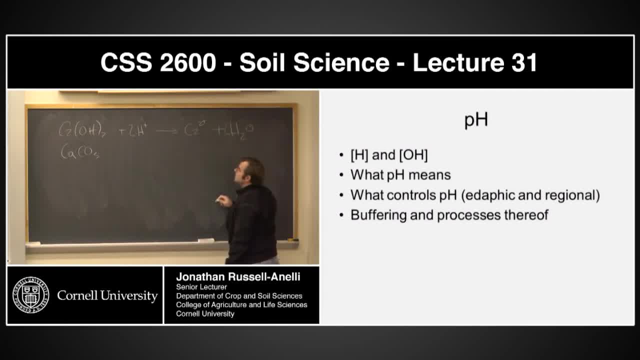 to make two water. Okay, So in essence, what I've done, this is coming in the solution. I've basically neutralized it. Okay, Now I'm going to keep putting protons into solution, And if I don't, 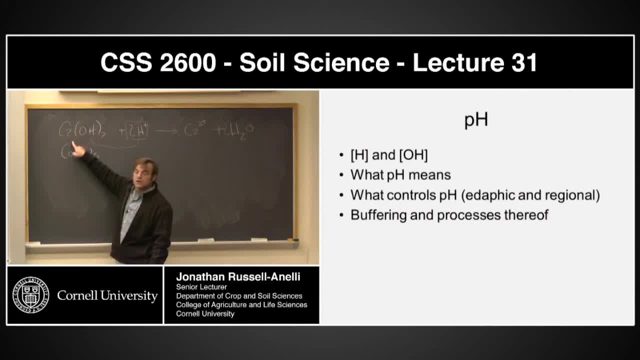 add more calcium hydroxide, sooner or later we're going to lose this buffering reaction, And at that point the pH is going to start dropping. Okay, The same thing is going to happen here with calcium hydroxide, calcium carbonate. 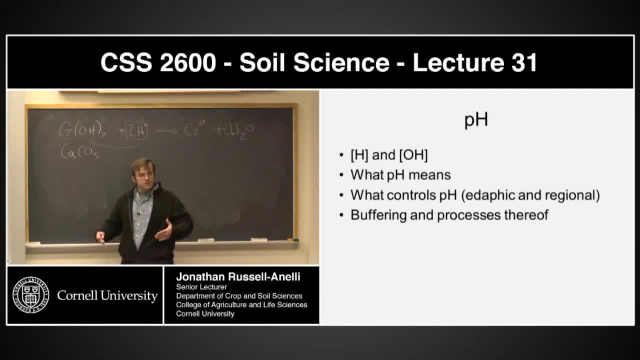 Now, generally, when we think about calcium carbonate- because we're thinking about this as a liming reaction in soil systems in the real world- when I add two protons in like this, I could be adding it as hydrochloric acid or something. 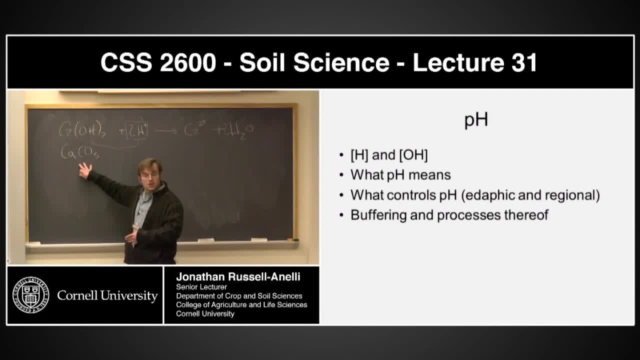 like that, But in all likelihood it's coming in as carbonic acid: Water plus CO2, making carbonic acid. Okay, That proton. now, this is not going to be a balanced reaction. That proton is going to react with this carbonate. 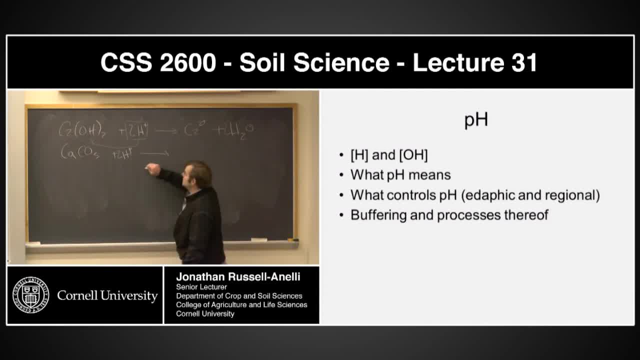 and basically do the same thing, and I probably should do this with two of them. Okay, What's going to happen here is these protons are going to react with one of those protons. One of those protons, because this happens to be carbonic acid.